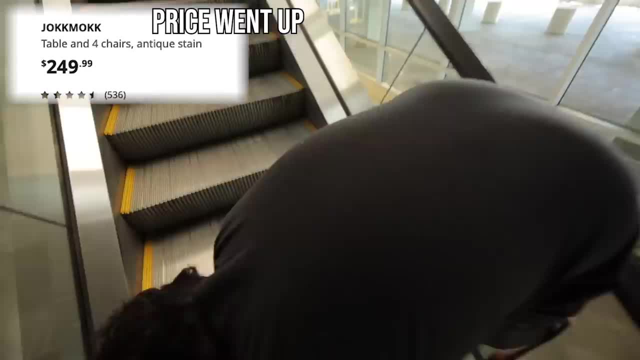 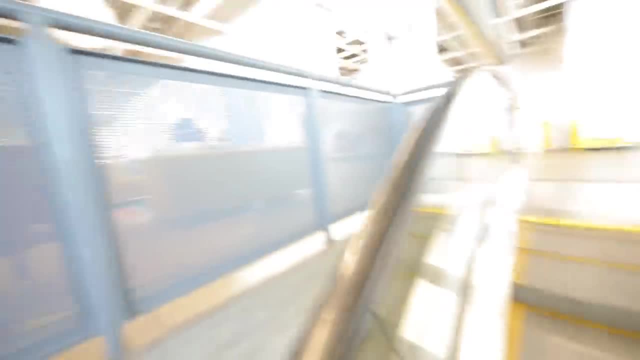 Let's go SHELFSITE at IKEA. Yeah, pre-IKEA stretching. Oh man, Not ready for this. Okay, so that's the table we're going to get right there. You see the blue circle right there. 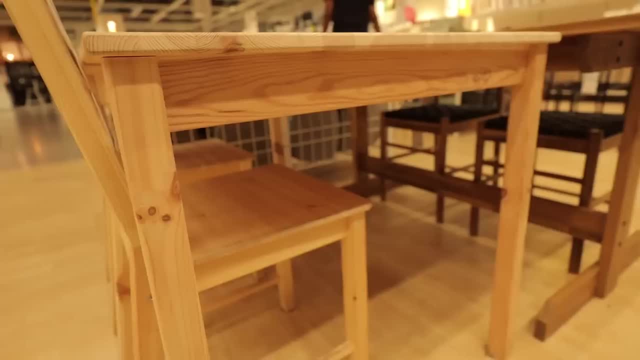 Yeah, perfect, We're going to turn that into a board game table. Uh-huh. Oh, this is the Jokemech. This is the one that you were talking about, Ashton. Ah, here we go. Yeah, The Jokemech. 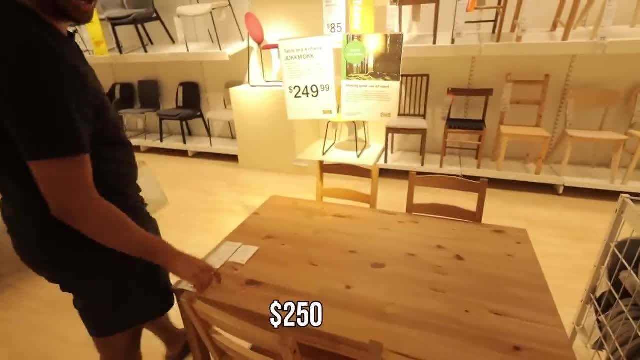 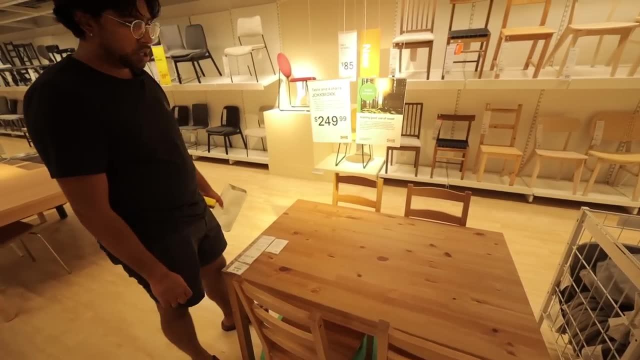 This is the table with the chairs: $250 bucks, But honestly I say we go for that one. It's the same size and you can just get the table by itself. Let's do that. Yeah, I just like the color of this more, but who cares? 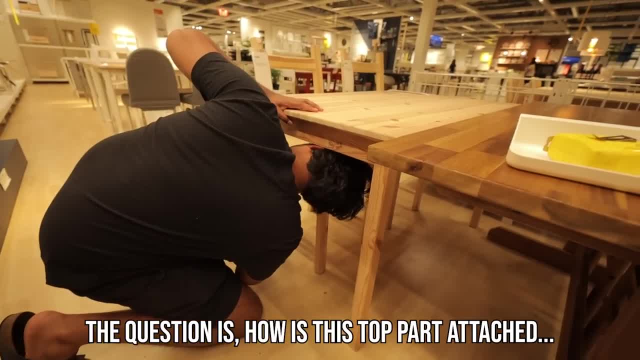 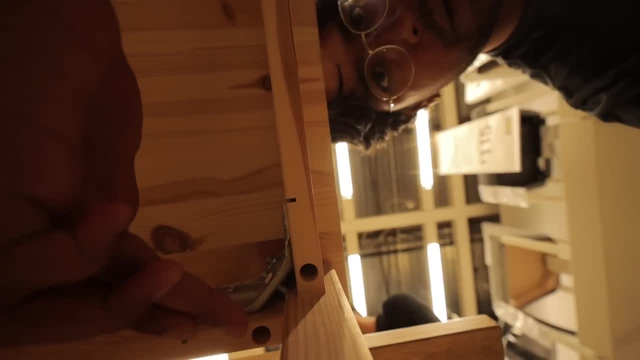 It is nice. We can always stay in that. The question is: how is this top part attached? If we're lucky, it's just attached through the through. a few bolts in these holes right there, right, So you can see this hole and you can see that hole right there. 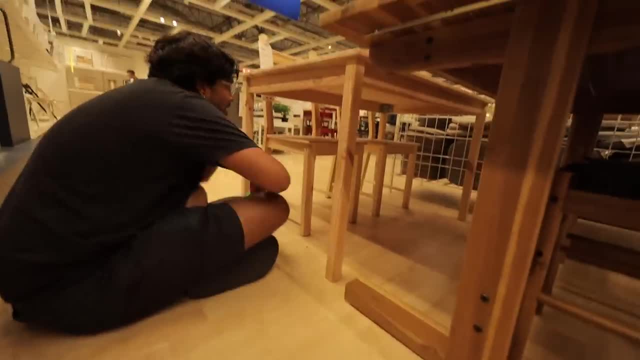 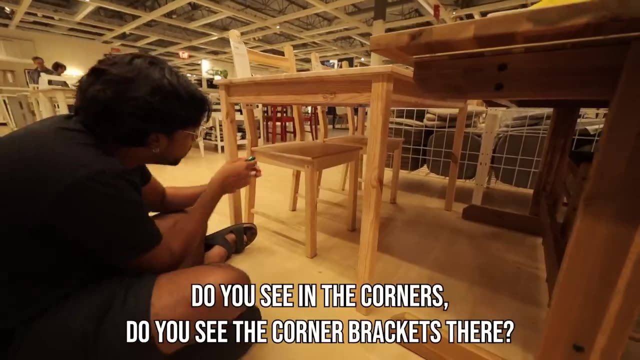 Okay, so here's the plan right now. okay, So, oh, the problem is these side pieces. It's going to look a little bit weird, potentially Okay. So, okay, if you take a look under here, do you see in the corners? 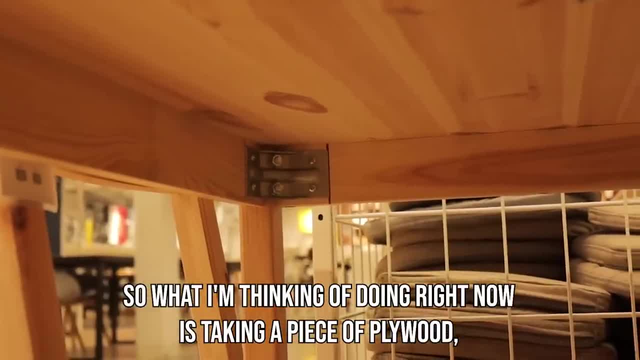 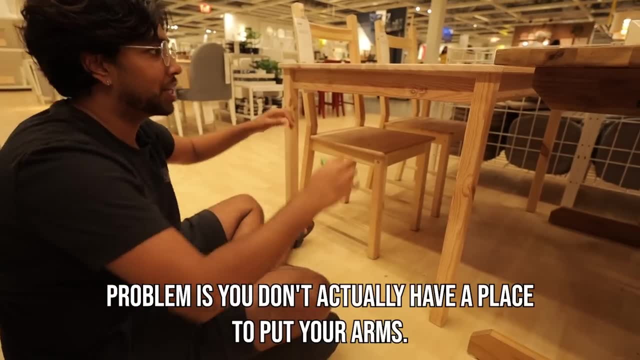 do you see the corner brackets there? So what I'm thinking of doing right now- taking a piece of plywood, slapping it on the bottom here and then just screwing it up to here. Oh okay, Right. Problem is you don't actually have a place to put your arms. 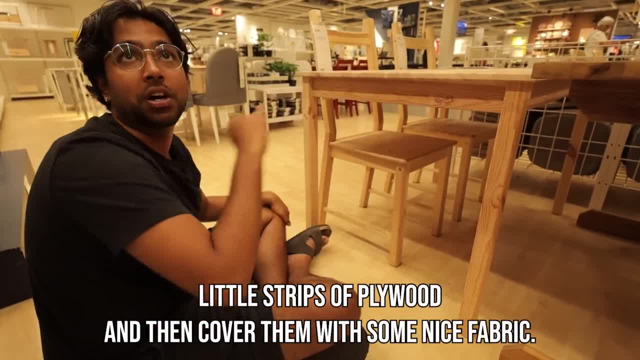 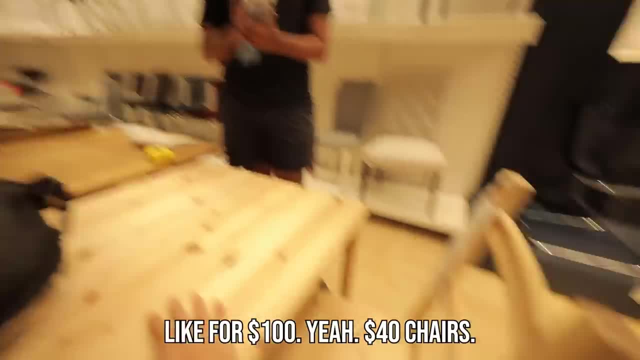 I'm going to basically just cut So kind of a sheet of little strips of plywood and then cover them with some nice fabric, Honestly pretty comfortable right now, as is Right, Like for a hundred bucks- Yeah, Forty dollar chairs. 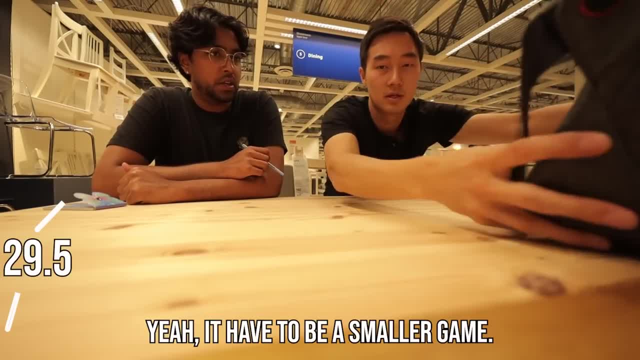 Playing a board game. we're going to be a little hunched on it, right, It'd have to be a smaller game, I think overall. Yeah, I mean, if we're sitting across from each other, especially this way, you have a lot of space. 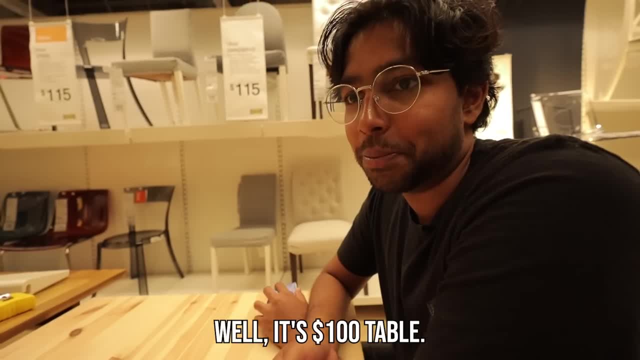 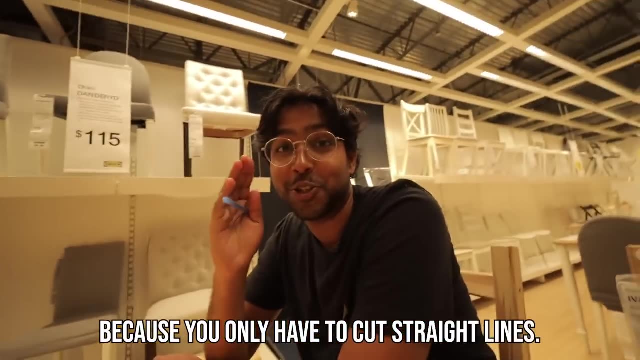 Yes, yes, This would fit a four-player game well. It's a hundred dollar table, so you take the limitations of what you get right. So much easier than building your own table too, Because you only have to cut straight. 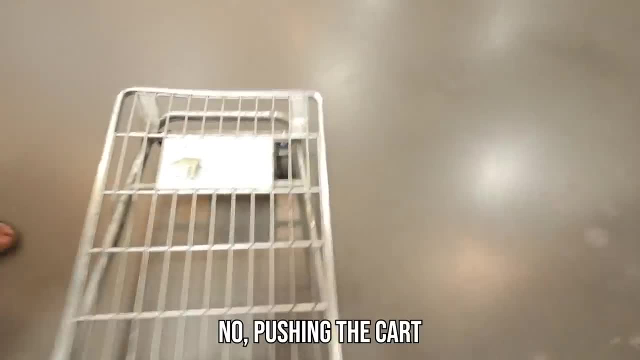 Straight lines the entire time. Yeah, let me. No, putting it in a cart is the most fun part. All right, okay, This is going to be hard to do with one hand, but we're going to see. Oh, do you want help? 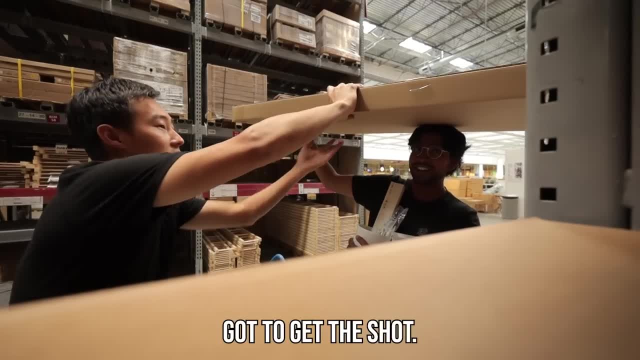 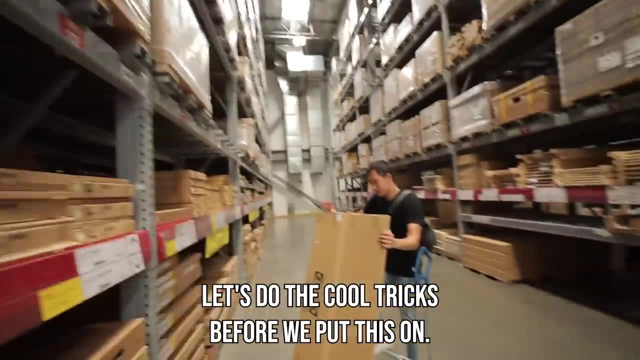 Yeah, I need some help. Yeah, here let me put the. Gotta get the shot. It's not light. You got this. Okay, It's 15 kgs apparently. What is a table? Let's do the cool tricks before we put this on. 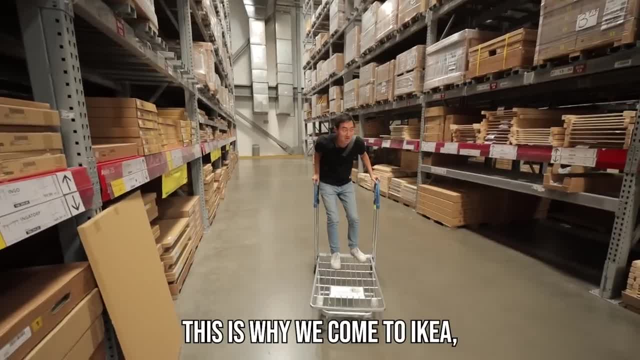 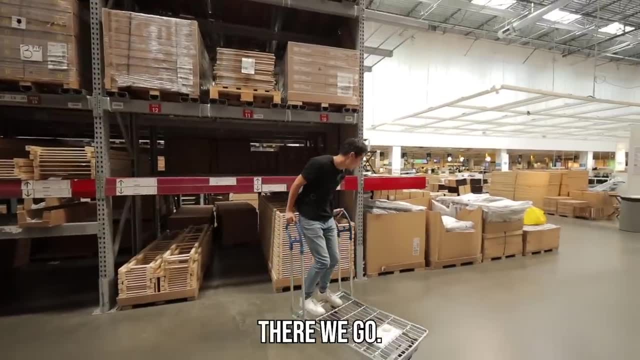 Yeah, Shelfside tricks. This is why we come to IKEA. Dude, this is actually really fun. Yeah, Why go snowboarding? Shoot which way? Ah, Ah, Ah, Ah, There we go. This is why we come to IKEA. 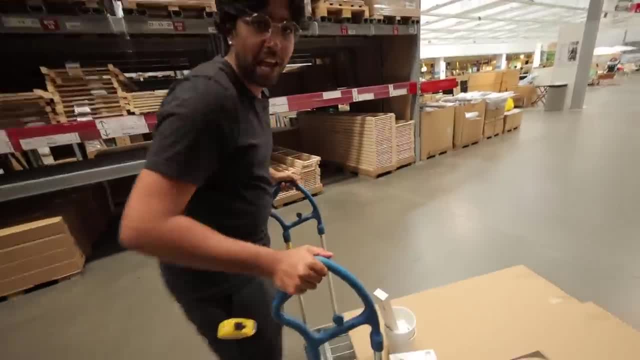 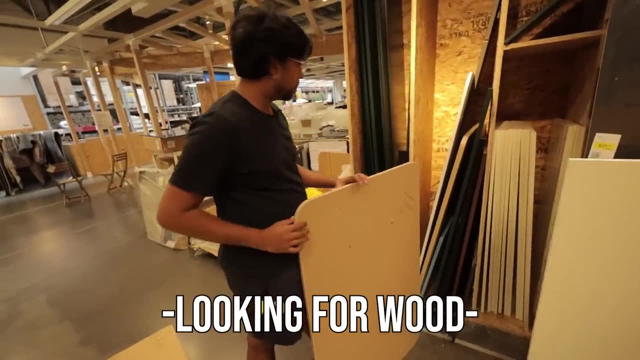 To screw around All right Day at IKEA. Ashton's not brave enough to do this, but I am, Oh you, rebel, Oh you know me. 75 is not worth it for what we're trying to do. You're a handy person in the handy person corner. 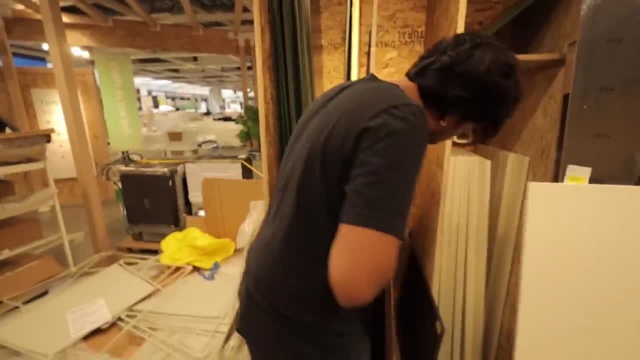 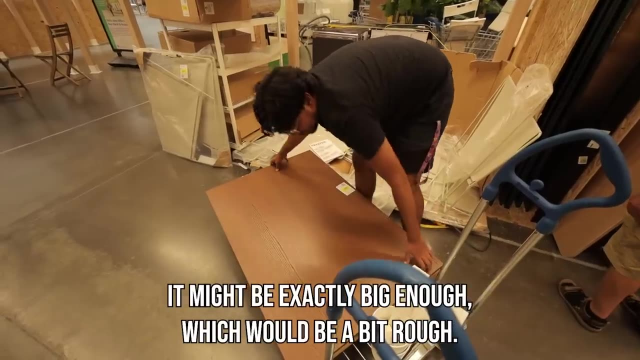 I got hands. Is that 20 bucks? Okay, this is 20 bucks, Okay. well, let's just make sure this is bigger than the table. It might be exactly big enough, which would be a bit rough. No, it's big enough. 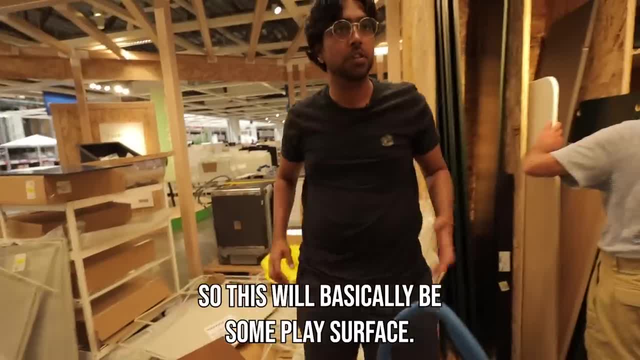 It'll be fine. Okay, so this will basically be some play surface, either the top entirely, and we'll chop up the bottom to use something. We'll use this for something. Okay, let's go for it. All right, let's do it. 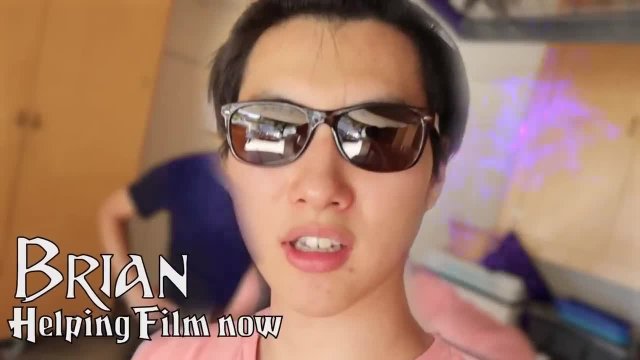 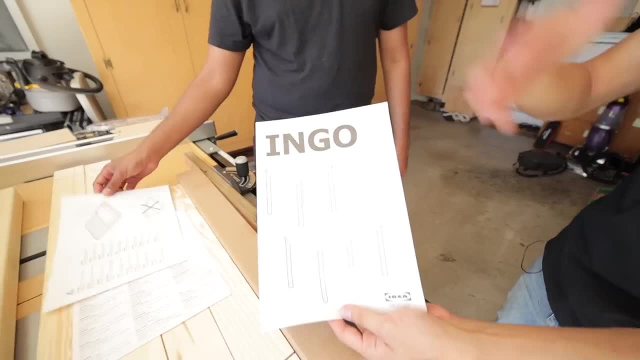 I'm your cameraman for today. My name is Brian and I don't know how to. Okay, so we have the Ingo table that we just got from Ikea. Ikea Pranav has unboxed it and we're going to assemble it and see what the heck happens. 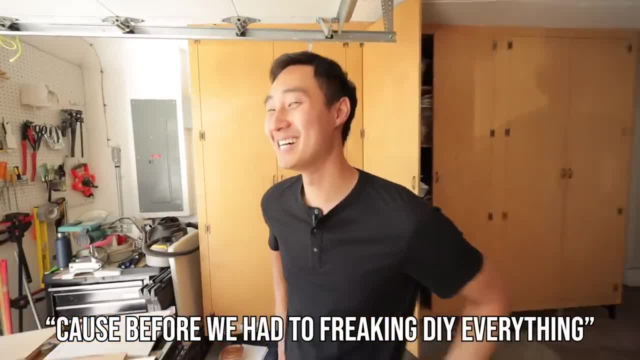 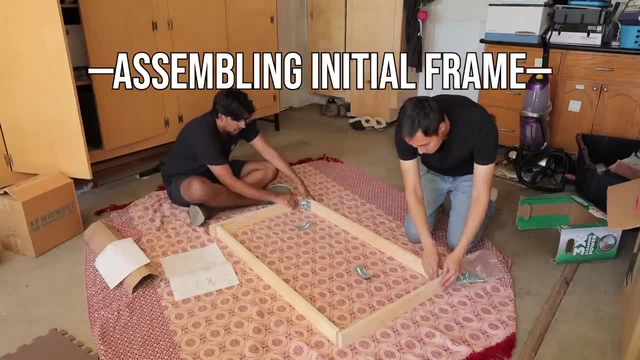 It'll be way easier than before, Pranav, because before we had to freaking DIY everything. This is very close to my face: Pranav is the main guy. Pranav is the main guy. You heard the man Just run up like this. 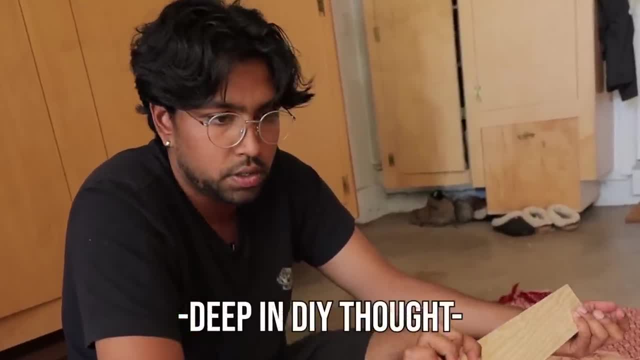 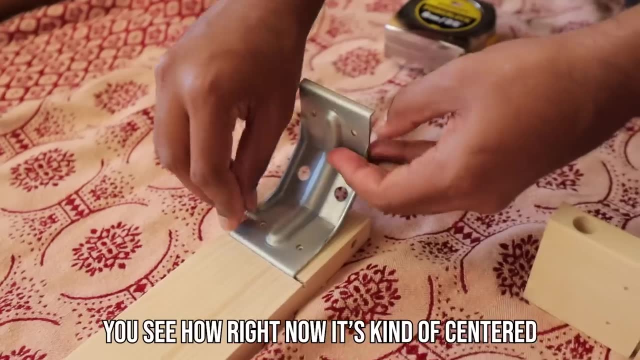 I want that one instead. No, I guess we could slap some. Oh yeah, because it goes. Oh yeah, because it goes. This is meant to interface with this corner mounting bracket. Do you see how, right now, it's kind of like centered right about halfway, like that right? 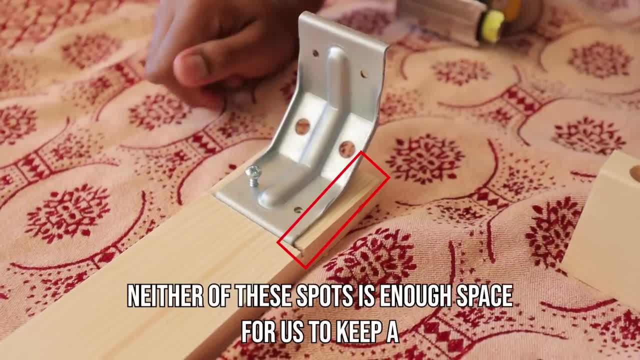 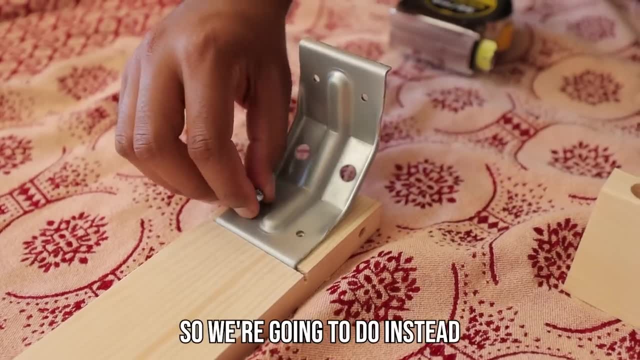 We don't want that. So what we actually want is: neither of these spots is enough space for us to keep a To like keep the base of the surface, like the base of the actual play surface. So what we're going to do instead is we're going to take these. 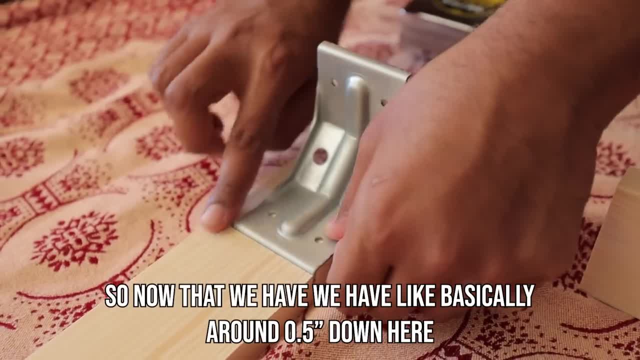 we're going to re-drill these holes up here. So now that we have like basically around half an inch down here, so we can lodge our play surface in here and actually drill through it on the other side, We should just drill like a tiny little hole. 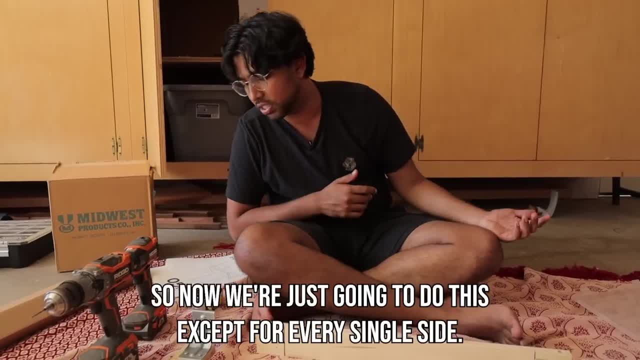 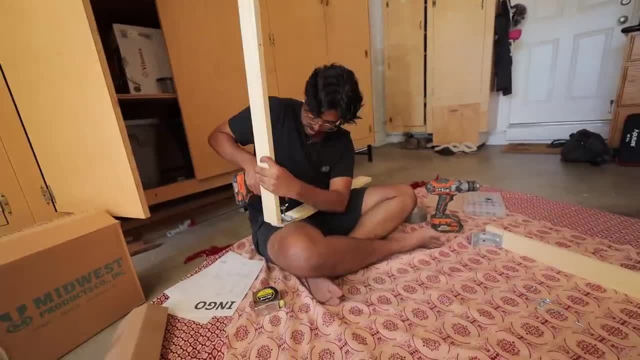 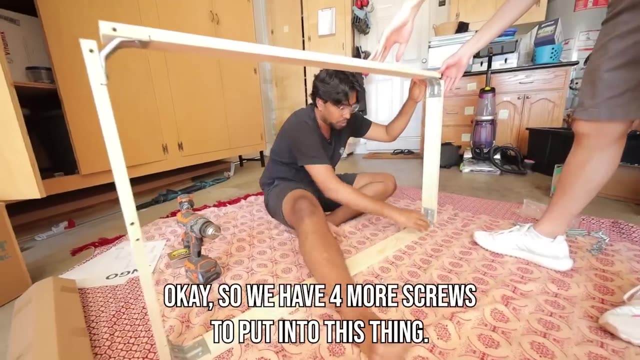 Okay, so now we're just going to do this, except for every single side. It's not ideal, but it's workable In this specific context. I mean, don't drill directly into your legs, Okay, so I got four more screws to put into this thing. 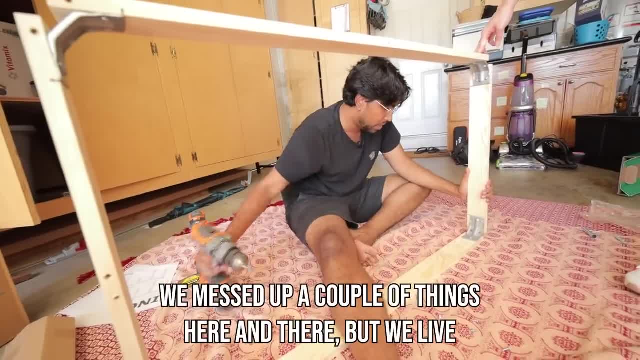 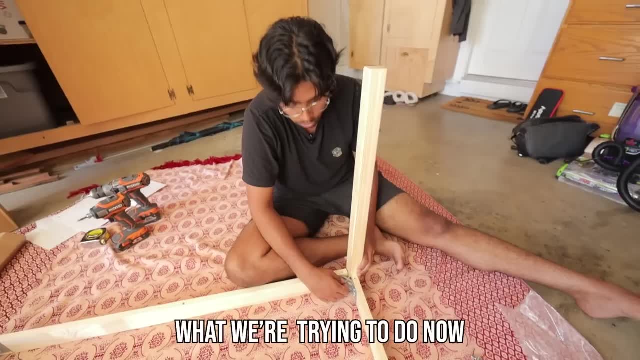 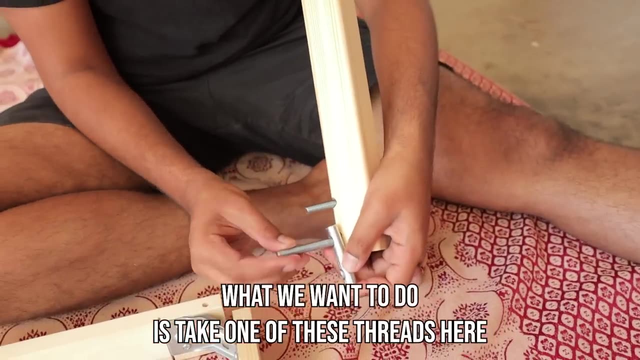 It's decently balanced. It'll be okay. We messed up a couple things here and there, but we live and we learn right. So what we're trying to do now is trying to get this into the right spot here, And then what we want to do is take one of these threads here. 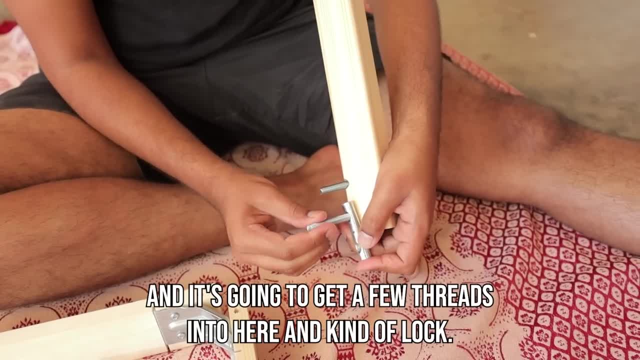 and then essentially just lodge it into here And it's going to get a few threads into here and kind of lock, and that's what we want. And then now we're going to put this mounting hardware on here, Put it all together. 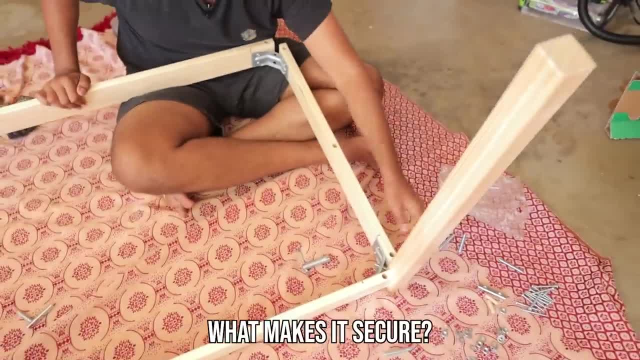 And there we go. That's our table, Holy cow. What makes it secure? It's because there's- look, there's two points of mount here, And it's also up like a bunch of Okay Plotted up against both of those edges. 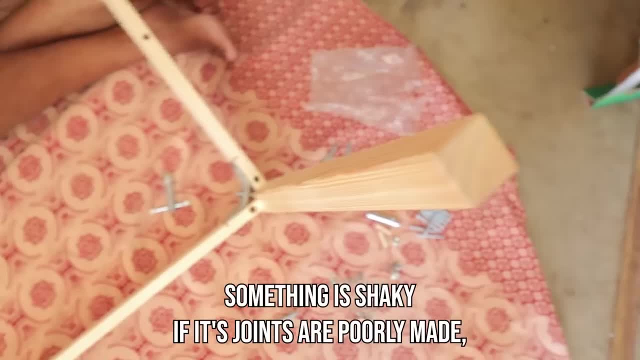 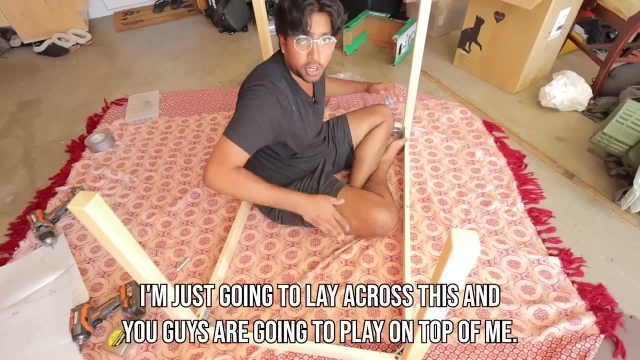 Do you see how that's all together? Yeah, we're good. Something is shaky if its joints are poorly made, but if the entire thing shakes at once, usually that just means it's not heavy enough. Here's our goal. I'm just going to lay across this and you guys are going to play on top of me. 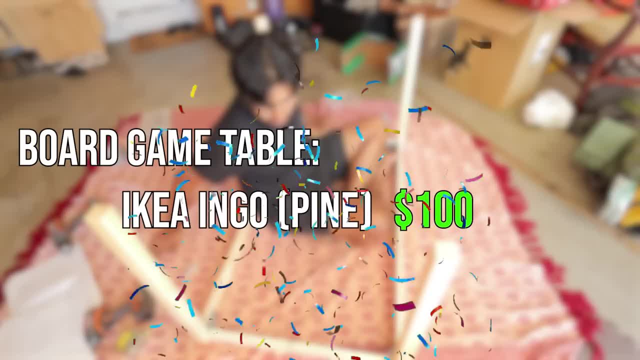 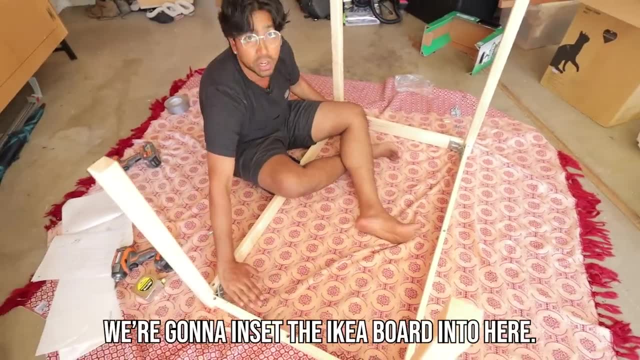 Yeah, Cool, Cool, Let's do it. Yeah, And then we're going to inset the board that we got from IKEA into here, essentially So that'll act as the bottom of our play surface. I don't know if you can even hear. 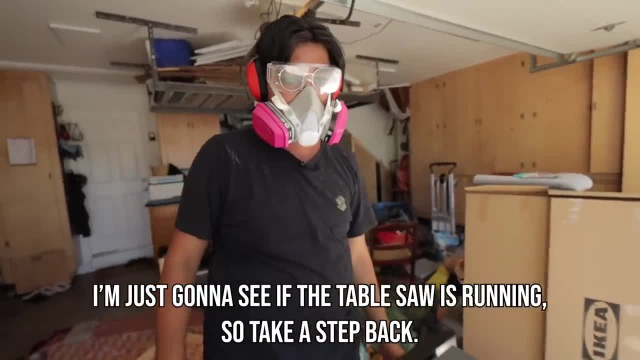 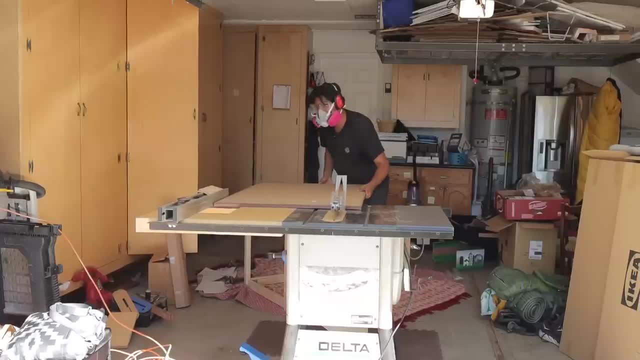 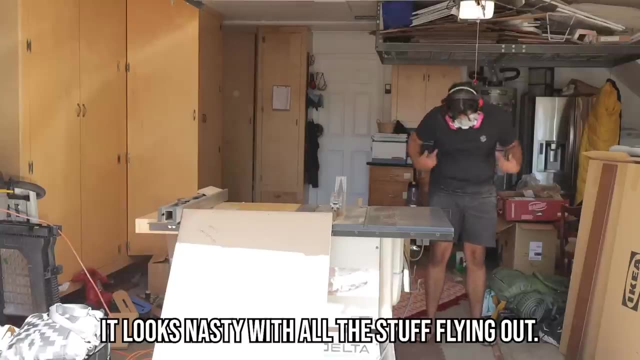 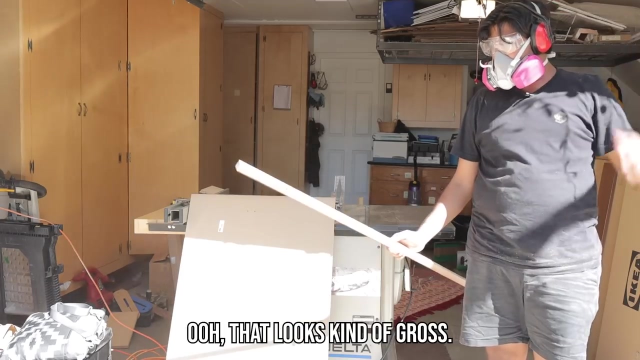 I want to be honest. I can actually. Okay, I'm just going to make sure the table saw is running so I can step back. It looks nasty All this stuff. It is really bad. Yeah, Ooh, That looks kind of gross. 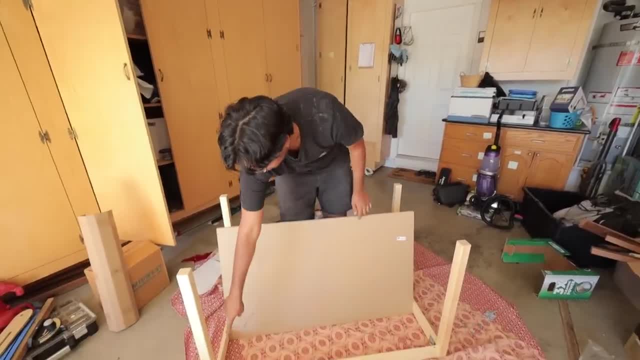 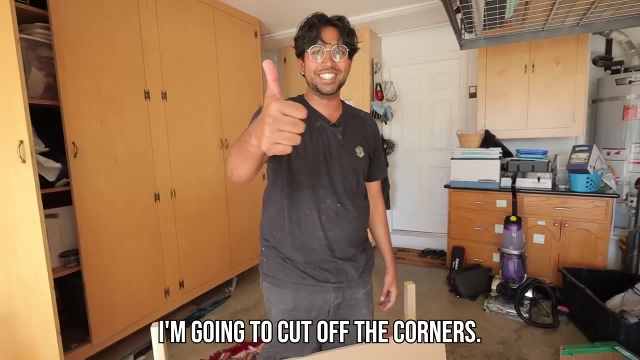 Fits perfectly both ways. Now all we have to do is make the corners fit in there. So what I'm going to do- And this is my really, really intellectual solution- I'm going to cut off the corners. Let's get up there. 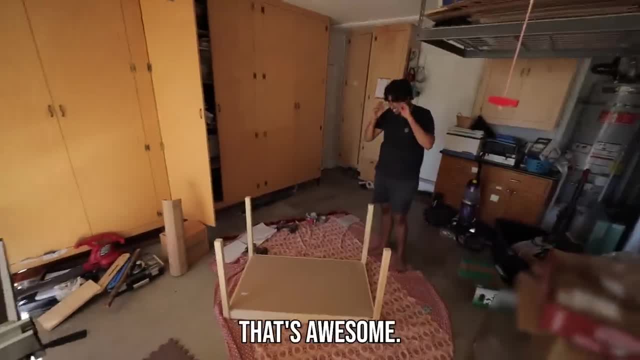 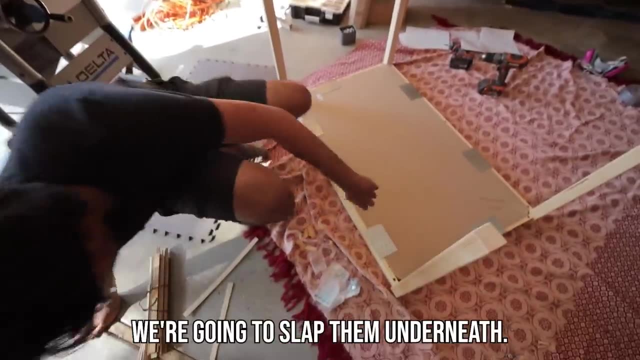 Cool. Look at that. Oh yeah, That's awesome. What the heck. It's still very secure. Wow, Wow, That's really strong. We're going to take these like 16th-inch spacers. We're going to slap them underneath. 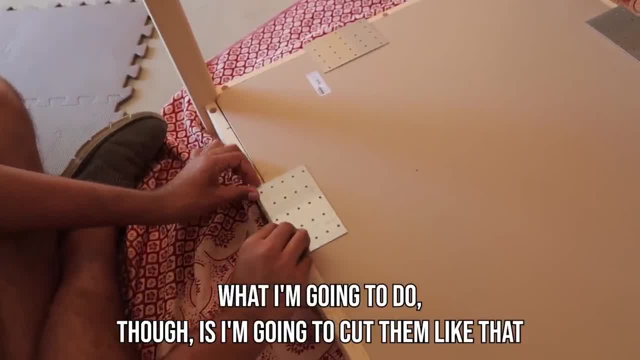 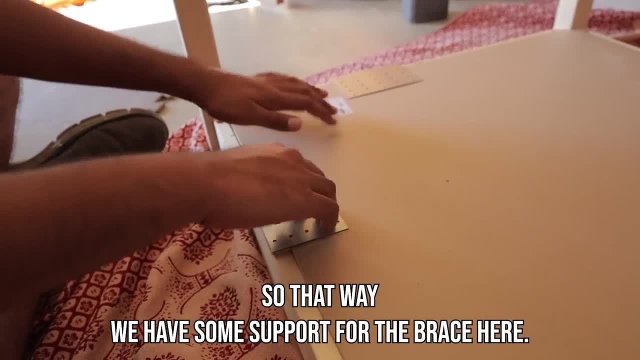 Cool. That's actually perfectly flush Cool. What I'm going to do, though, is I'm going to cut them like that, Run some screws through here, and then we're going to do that the whole way around, So that way, we have some support for the brace here. 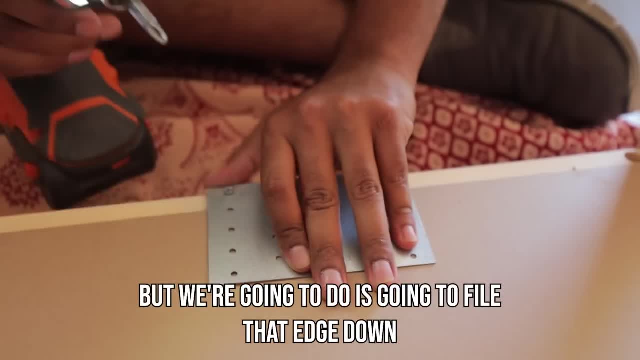 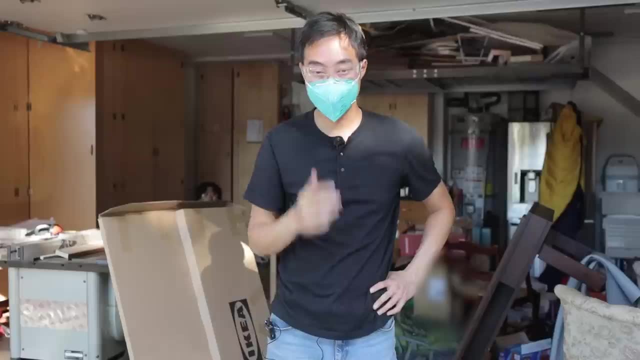 Now this actually juts out a little bit. What we're going to do is we're going to file that edge down. My left, or your left, My left? Oh okay, Are you done yet? Are you hot? I think we have some time left. 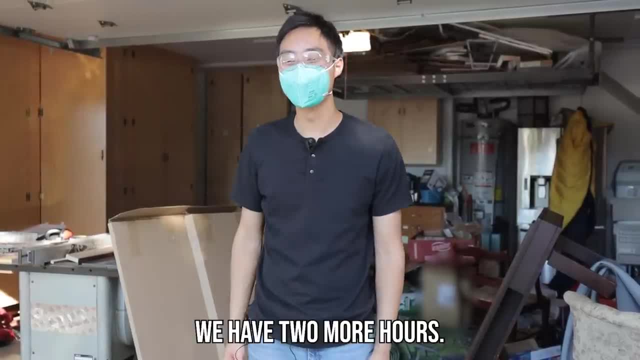 We have like two more hours. Oh Okay, We have two more hours. Two more hours, Yes. How are you feeling? Not bad, It's getting cooler. The sun is setting. Pranav's hard at work. 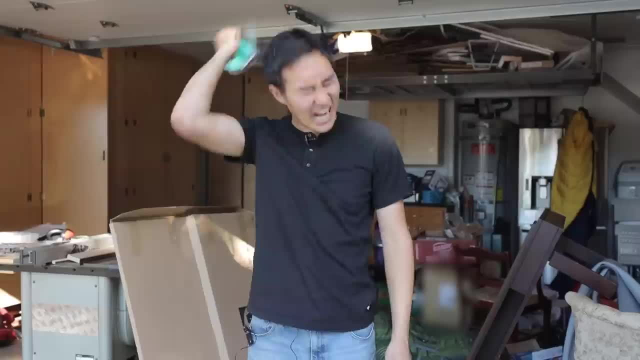 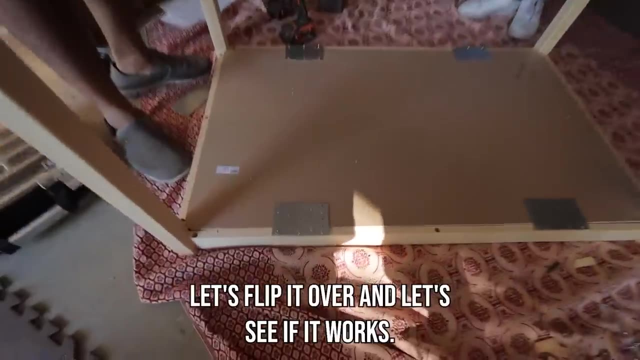 I just finished vacuuming, So it's all good. Ah Yeah, Feel good. We have metal braces that have attached this and mounted this properly. Let's flip it over and let's see if it works. Okay, All right. 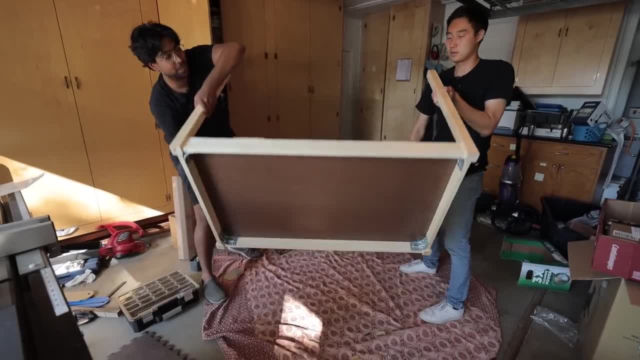 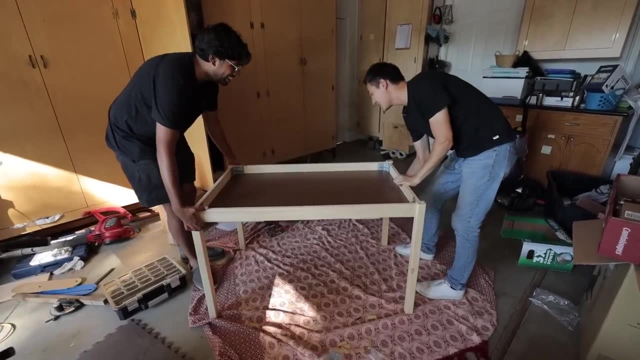 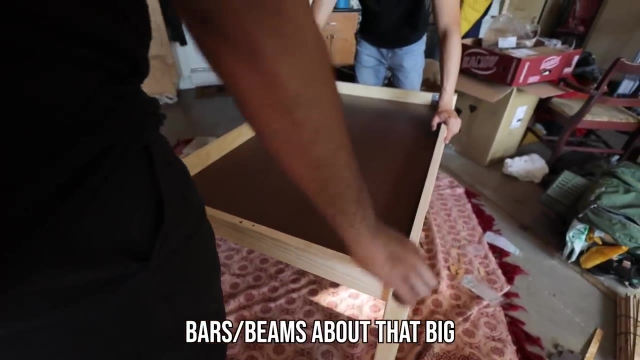 Ready. You have a twist in your arm. This is actually not that heavy, Whoa. Look at that. Okay, That actually looks pretty sick. Okay, That's pretty stable. Look at that, dude. Look at that. What we're going to do is cut bars, beams about that big, and we're just going to butt. 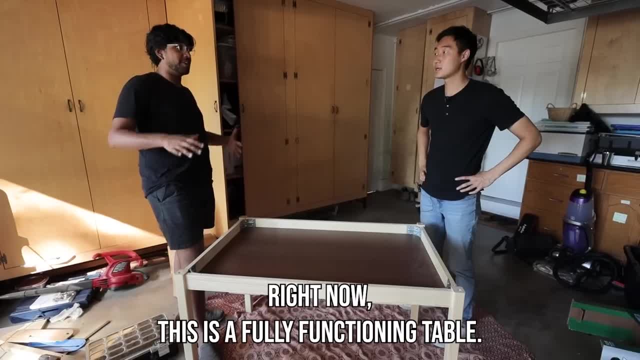 them up against each other, I see, And then we're just going to screw up into them. Right now. this is a fully functioning table. Yeah, Do you want to just try putting it on the topper? Just the topper. 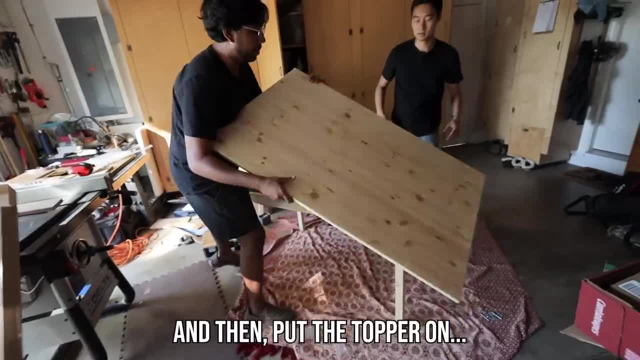 Sure, Let's put the topper on, So we can set up a little board game in there and then put our topper on And whoa, Look at that. And then this is going to be another like three quarter inches higher. 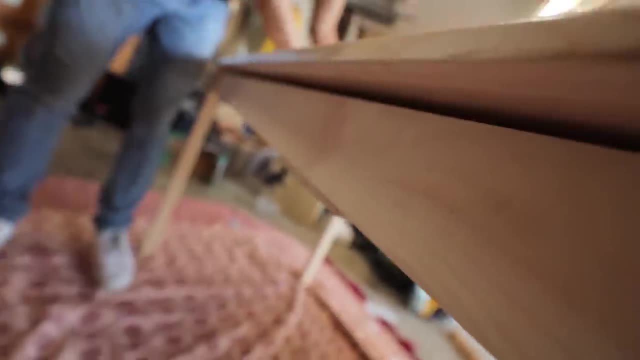 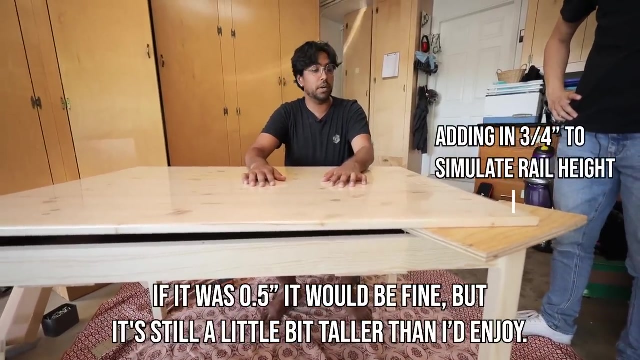 So that's going to be the one little stick out part, But that's okay, It's not really going to bother you too much, Okay. Okay, This is honestly a little bit taller than I'd like, Which is annoying. If it was half inch it'd be fine, but it's still a little bit taller than I'd enjoy. 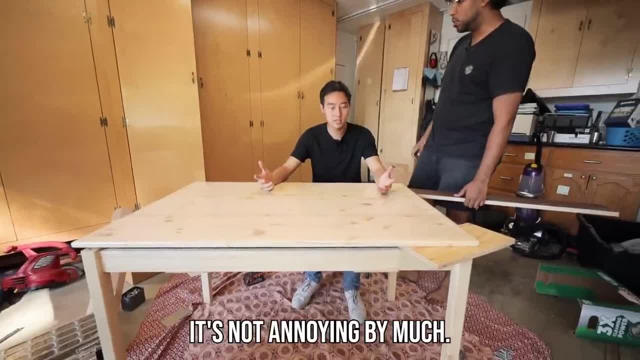 honestly Okay. That tall though It's not annoying by much, I could see myself eating dinner on here, no problem, Yeah Right, Yeah, Okay, cool, That's legal. What we have here is called a sacrificial fence. 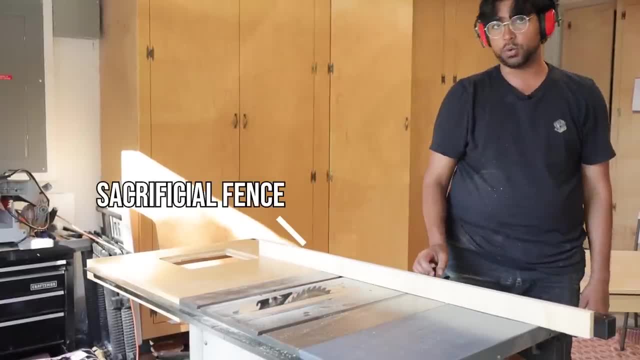 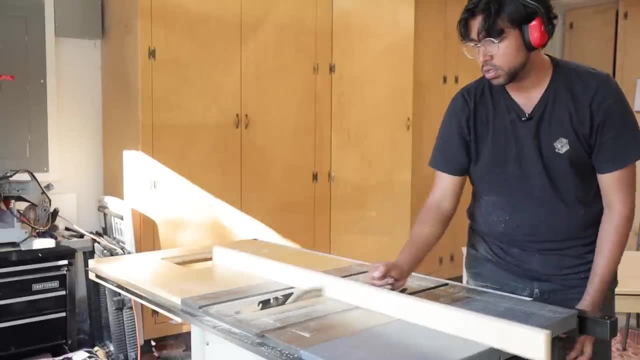 We're going to be trimming down those pieces that you see to the right thickness, So I'm going to run one pass real quick right now. So now we can measure off of that, We can measure off of this, because this is exactly where the saw blade starts. 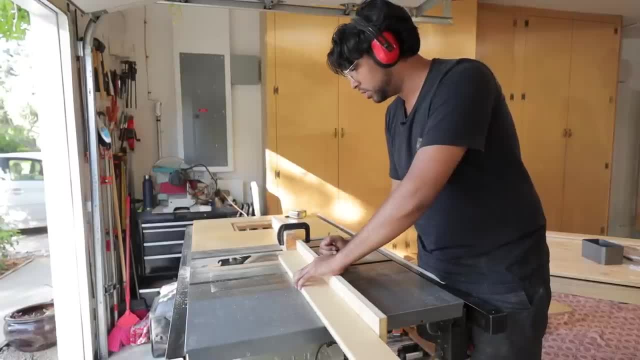 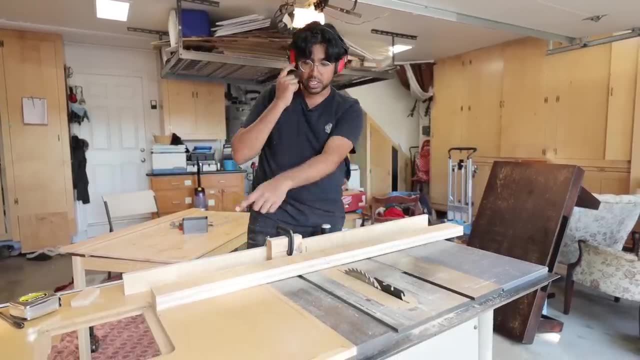 We can measure off of here to there for exactly the length that we need. These are going to be our armrests on the long side. We'll cut down the corners so they don't poke you a little bit, And this should be totally fine. 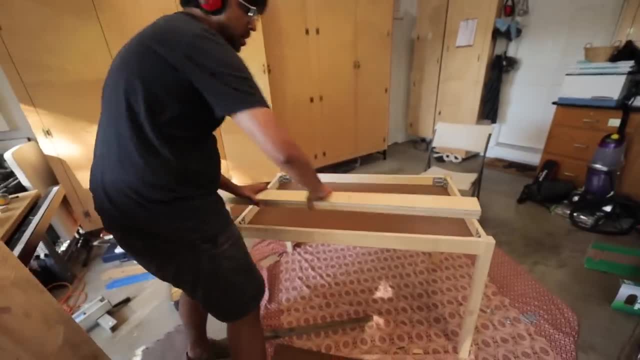 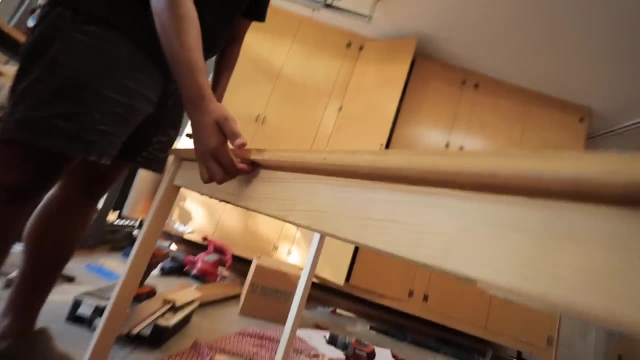 Internal play surface. Let's grab. thank you these two bits. So this goes right here. Our only problem right now is: let's look right here. Do you see this little gap right there? We have to find some way of filling that. 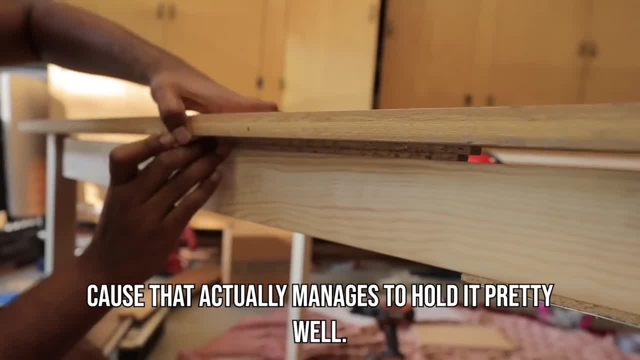 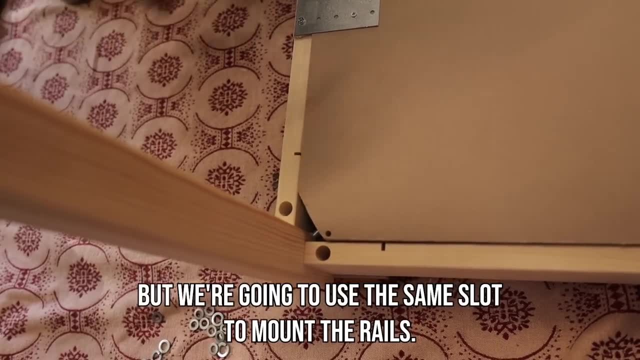 You can try something like this guy, because that actually manages to hold it pretty well. He already has these. These are to mount the actual tabletop, But we're going to use the same slot to mount the rails. Gnar, Look at this, Ashton. 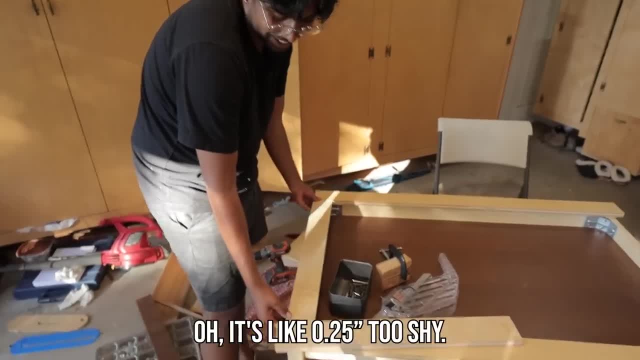 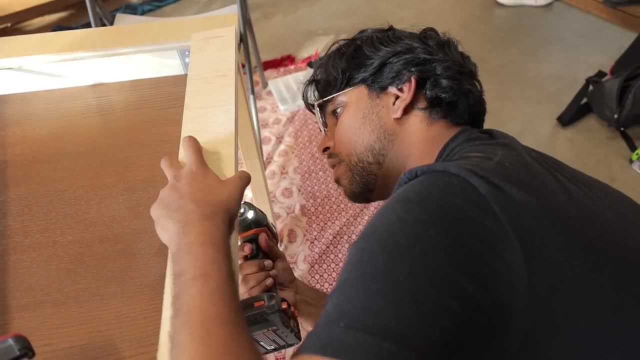 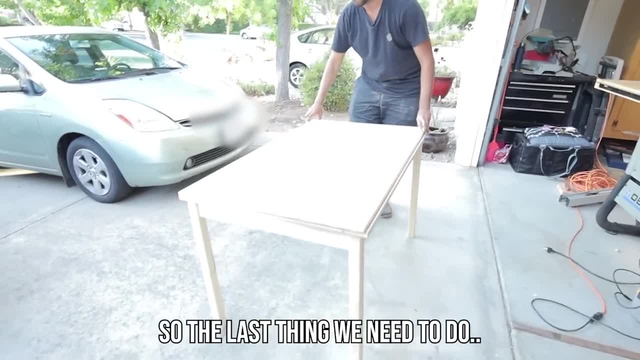 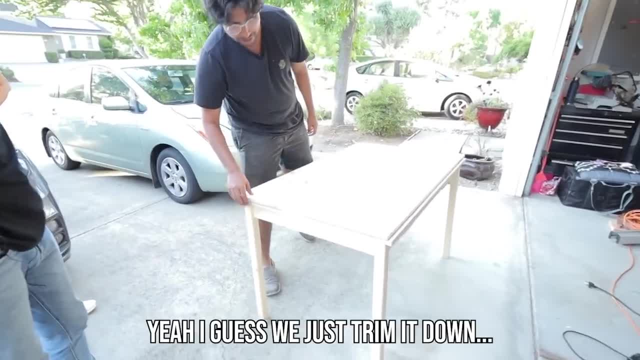 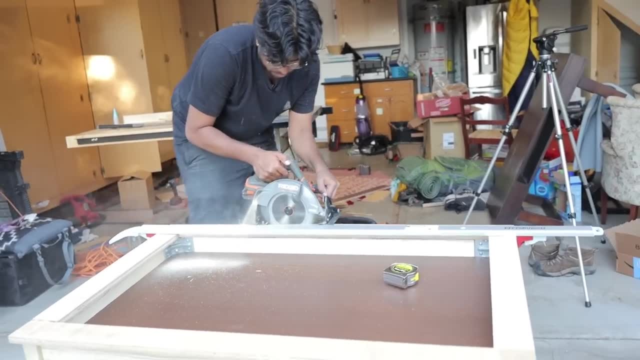 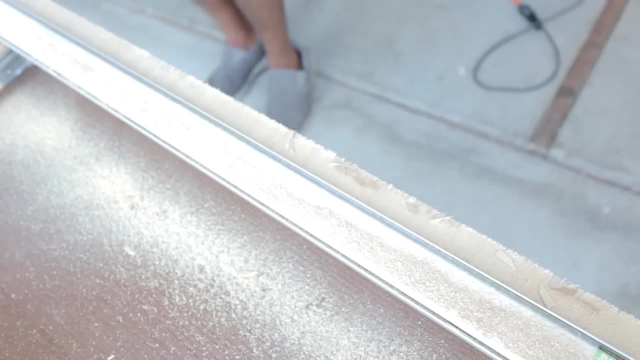 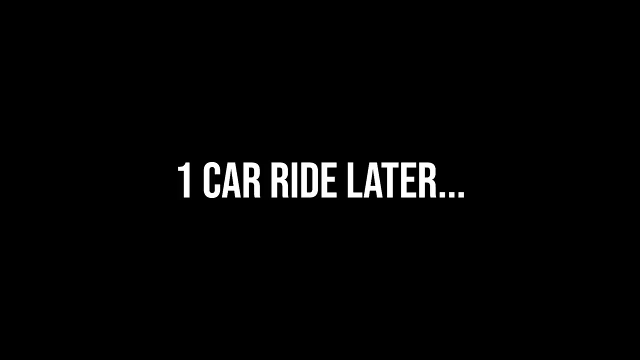 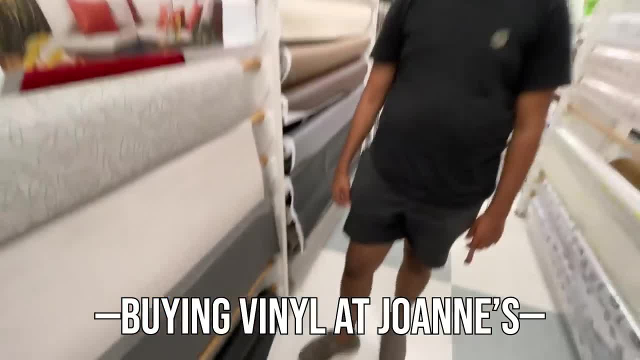 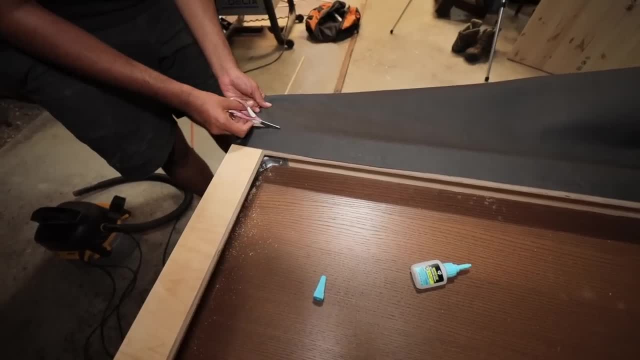 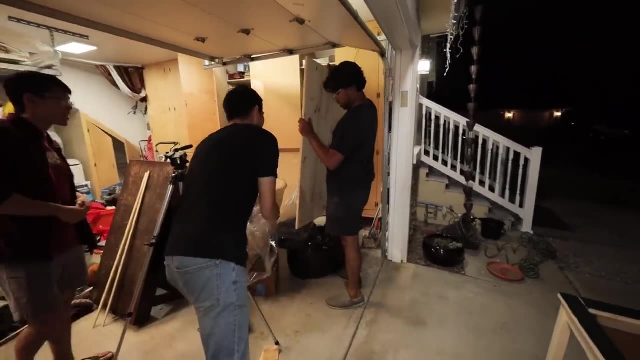 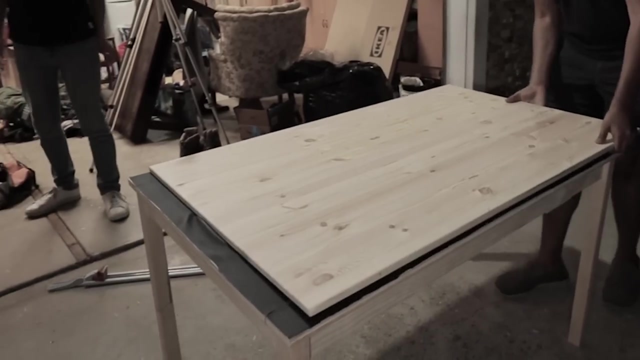 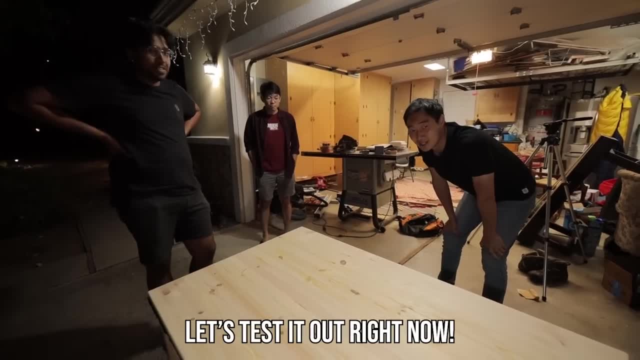 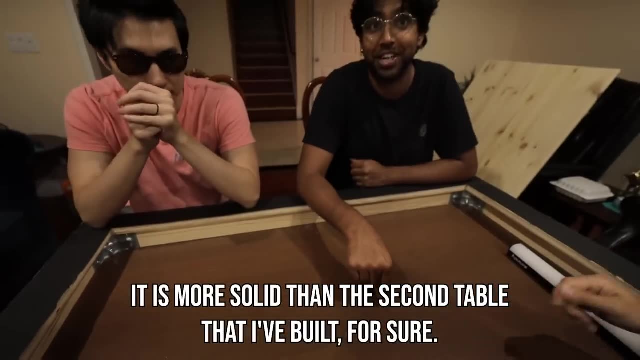 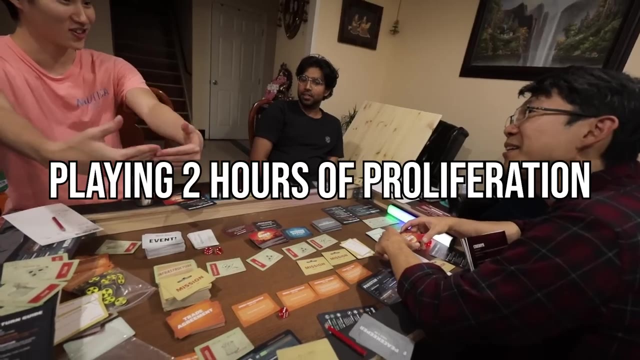 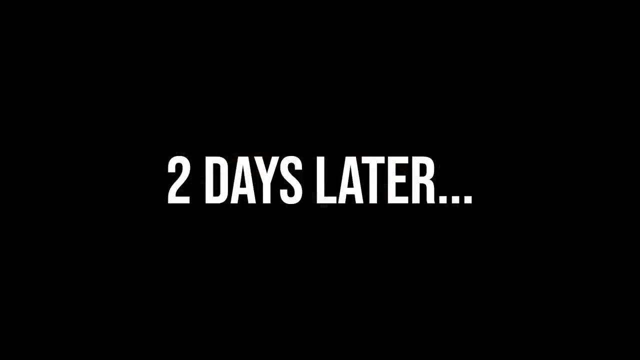 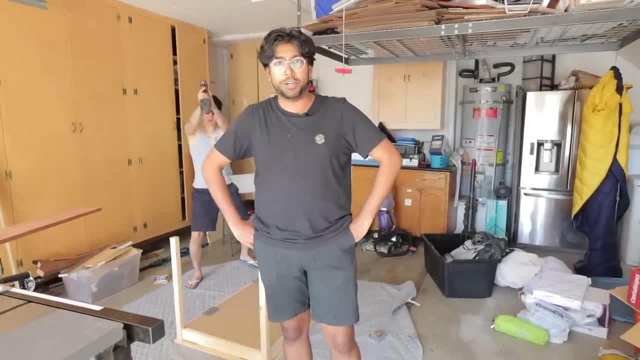 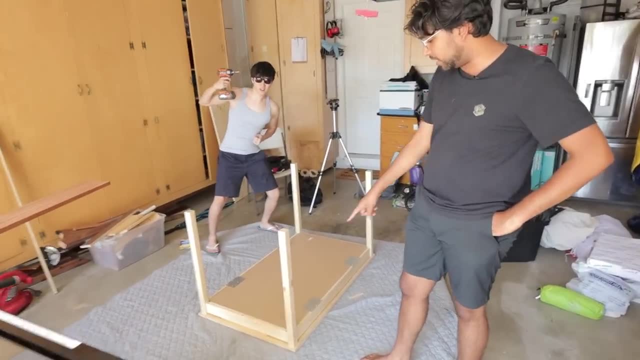 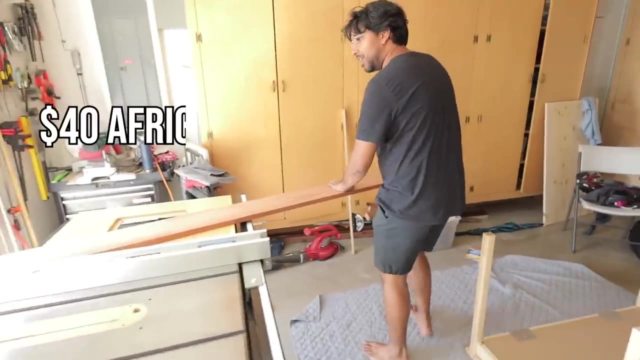 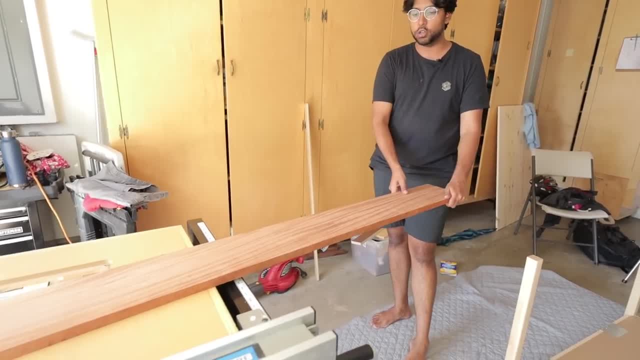 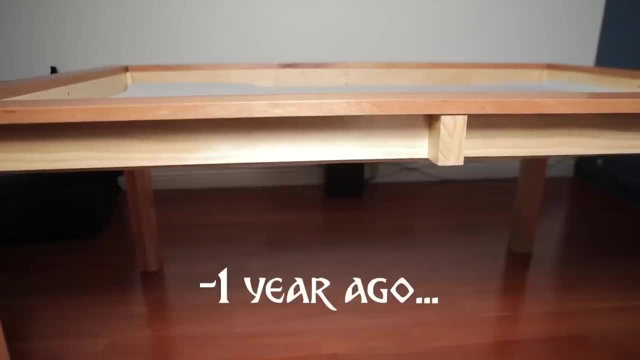 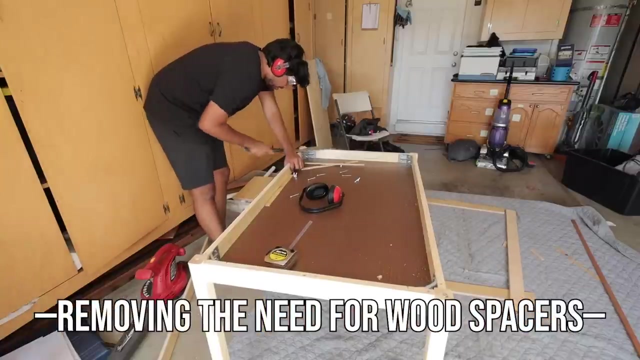 It's about. it's just under an inch thick and it just looks absolutely gorgeous. So this actually will look almost identical to the second board game table that I made, except this is sturdier and a lot cheaper. So that's on there. 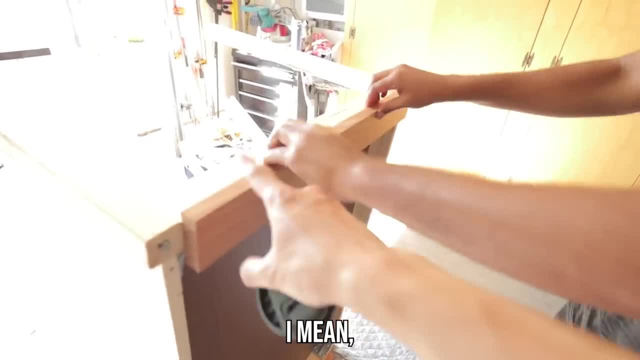 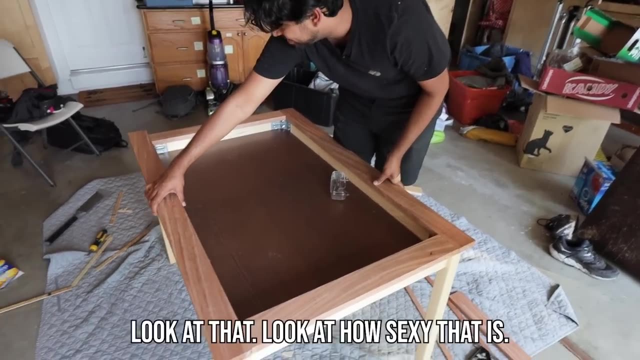 Yeah, it's on there. Wow, I mean: Okay, Oh, this looks so nice now, Yeah right, Wow, Yeah, Holy cow, Look at that, Look at how sexy that is, Wow Right, The price has just doubled. 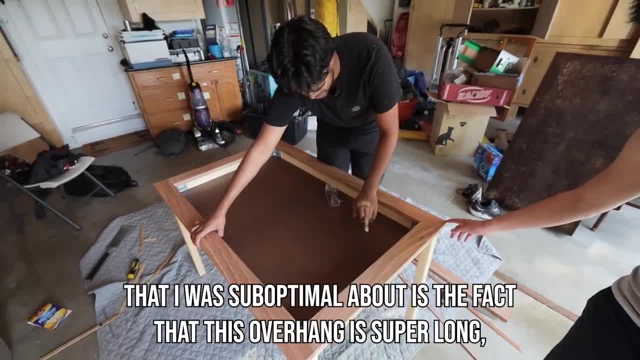 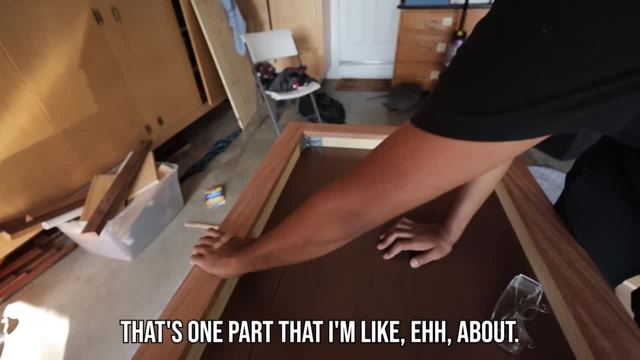 I mean, like the value. The only thing that I can think about this, that I was like suboptimal, is the fact that, like, this overhang is super long, but this overhang right here is relatively short. You see that That's one part that I'm like eh about. 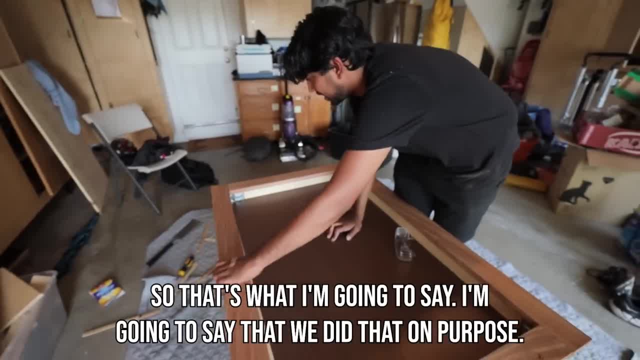 but also it means we have more play space this way. So that's what I'm gonna say. I'm gonna say that we did that on purpose, Got it. But these I just carved out a little bit. They're not perfect. I'm gonna sand them down. 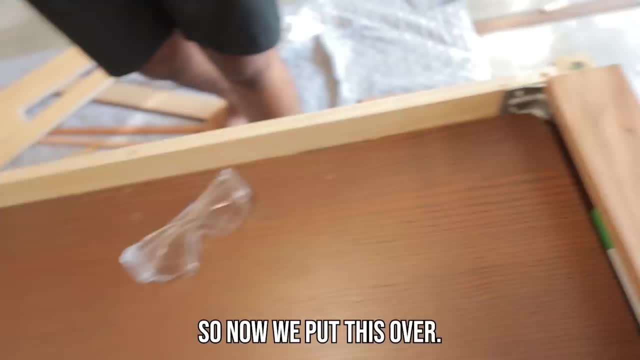 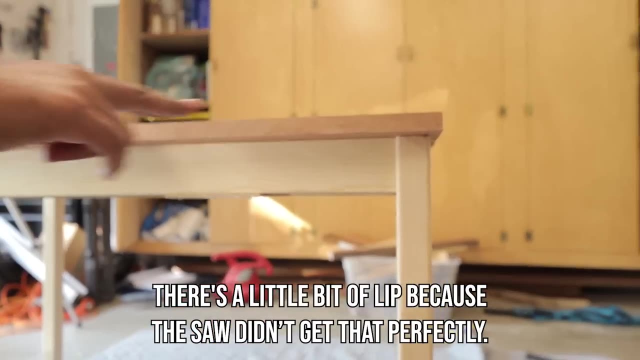 and then these will fit around here, which they do. So now, if we flip this over, it is perfectly flush right. there There's a little bit of lip because the saw didn't get that perfectly, but it'll all get fixed in post, so that's okay. 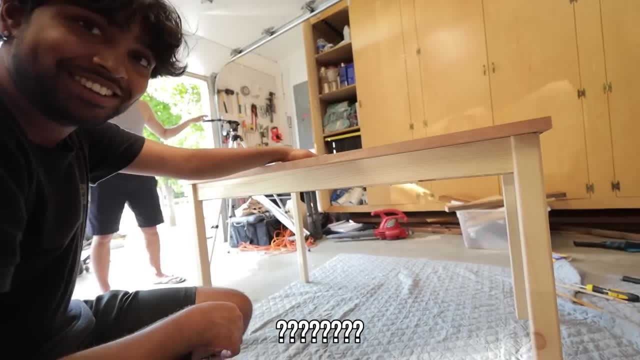 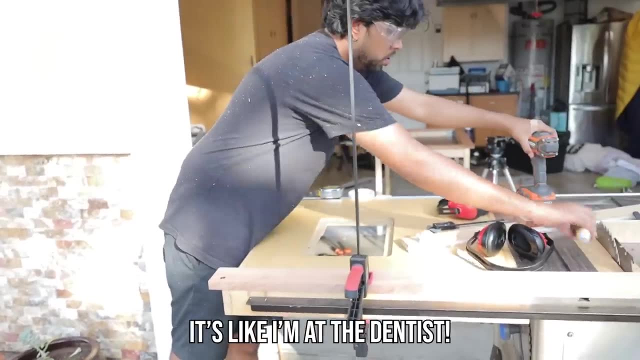 What Huh, Right, Ashton. Wait, what Right, Ashton, You're gonna fix that in editing, right? Uh no, It's like I'm at the dentist. Yeah, yeah, I'm gonna do this to your teeth next, Ashton. 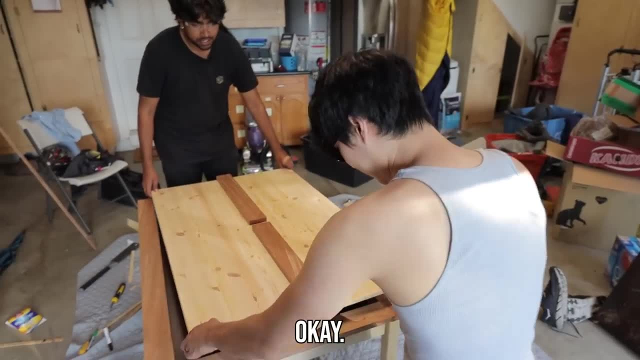 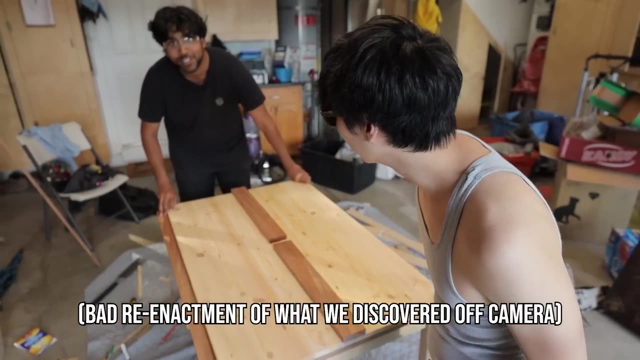 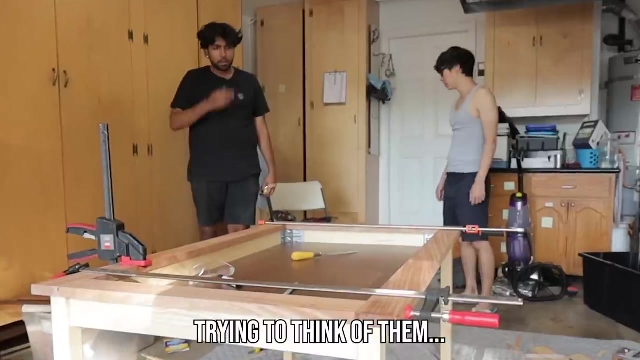 All right, let's test it, Okay? Oh, fuck, Shit, Pranav. So we're about two inches off, Pranav. There are solutions to this. I'm trying to think of them. We forgot to account for the topper. 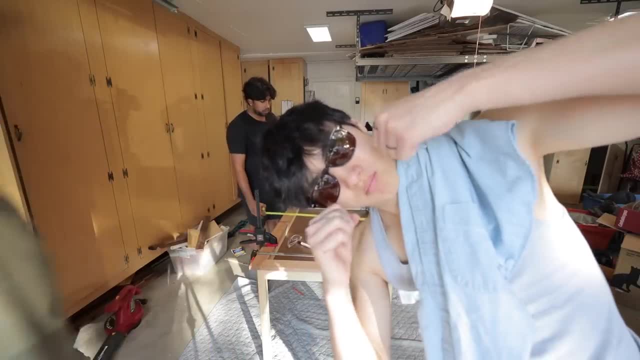 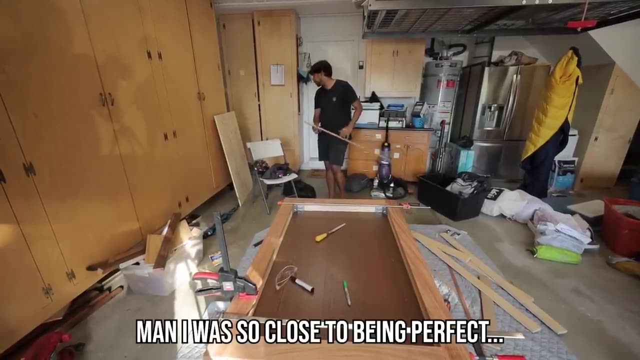 We don't have what We don't have enough. I see That's unfortunate. I know so close to being perfect, It's fine. it's fine, It's just a design feature. yeah, Yeah, why don't you just cut that in half? 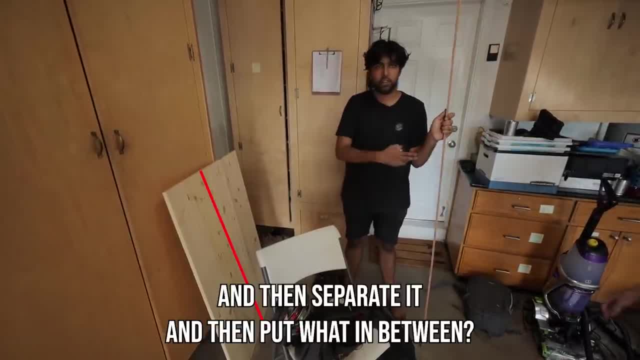 Cut that in half this way, maybe, Yeah, And then separate it and then put, like, what in between? Put this in between, maybe Yeah. Oh yeah, that's a good idea. Yeah, because it's rounded right now, right. 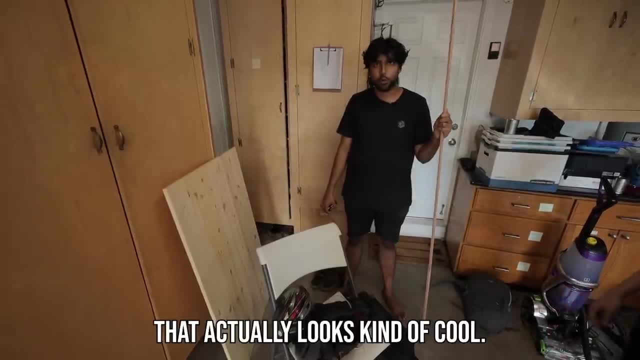 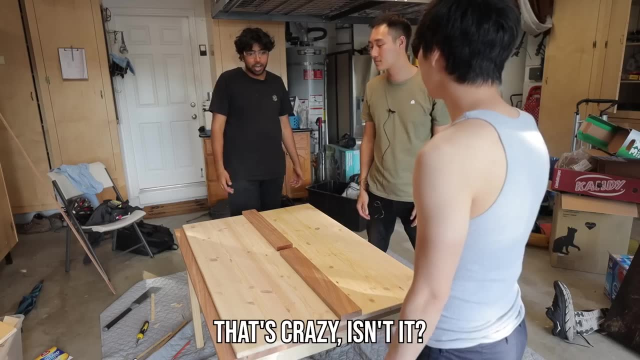 One mahogany strip in the center. Mm, that actually looks kinda cool. That actually is pretty smart, Okay, yeah, yeah, yeah, let's do that. okay, We actually intended to do that this entire time. It's crazy, isn't it? 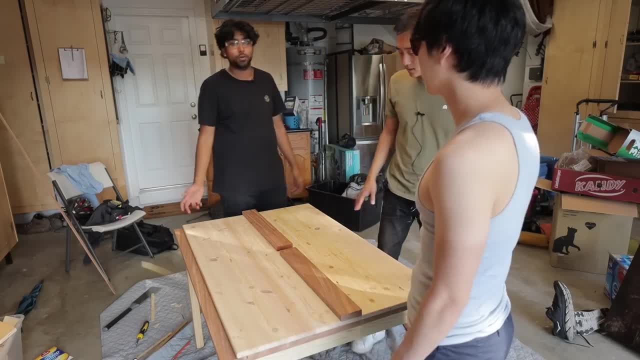 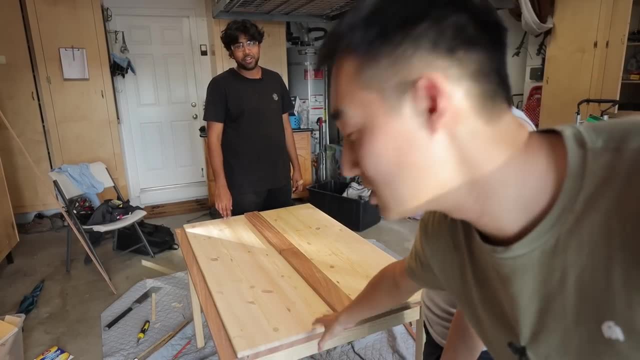 What we're gonna do is we're gonna cut the topper in half and then we're gonna put a little wood accent for it. What is this doing? This is our wood accent. Oh, This is the true DIY now, because this Ikea wood, this came as one piece. 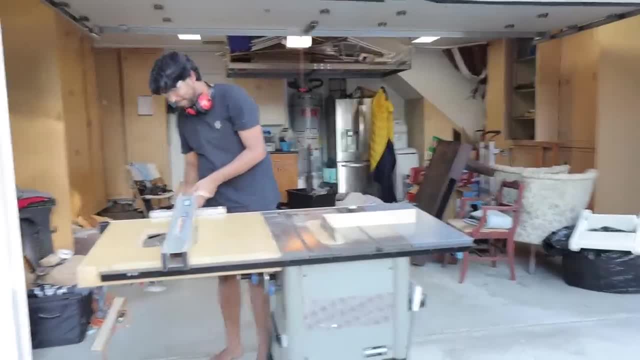 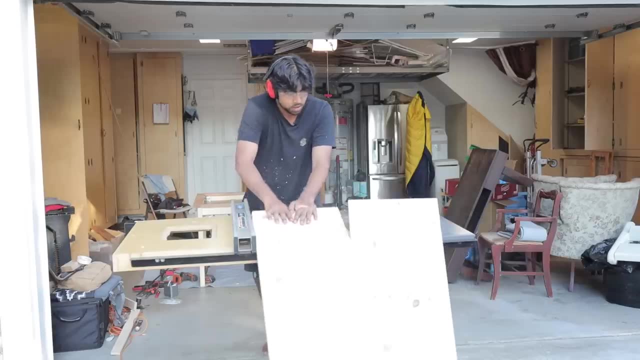 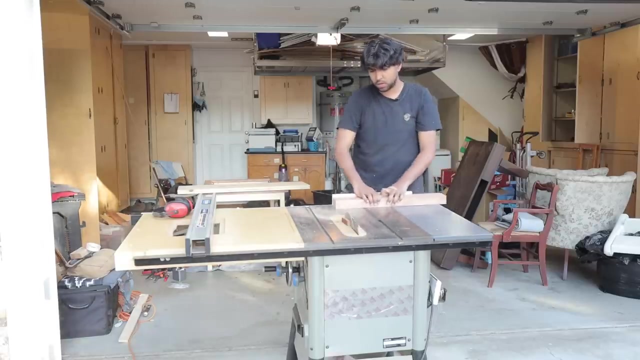 now we're cutting it in half. Yeah, I came. I saw I messed up. Ready, No, going back from this now. Cool, These two are the same length. we're gonna chop a bunch of one-inch strips off of them. 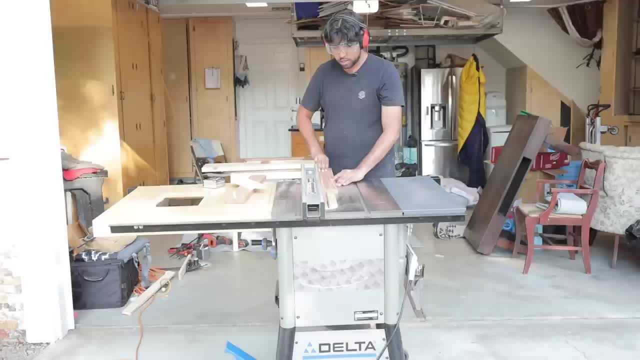 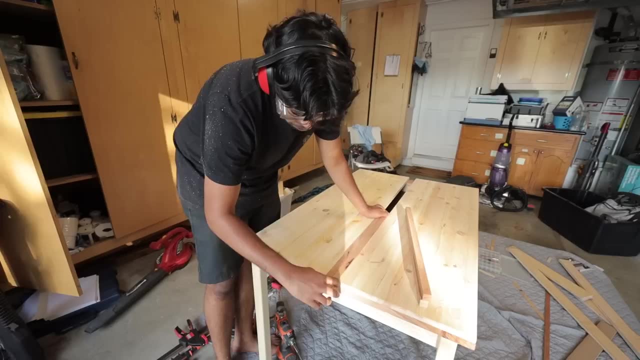 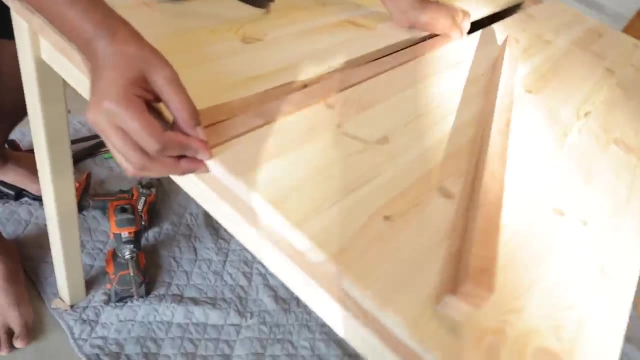 What's 2.75 by three? What's 15 sixteenths? Okay, perfect, look at that. This mahogany is a bit thicker than the pine here. It's like a good quarter-inch raised. I think It'll be annoying for big board games. I think, though. 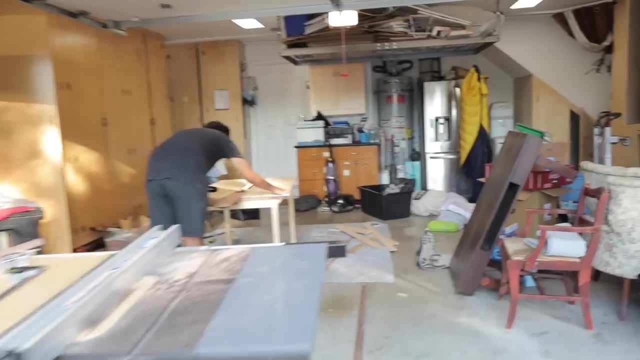 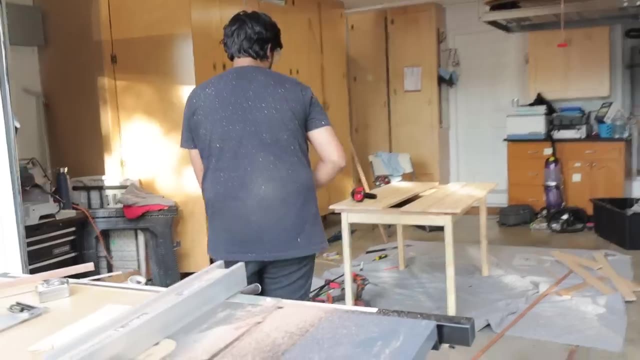 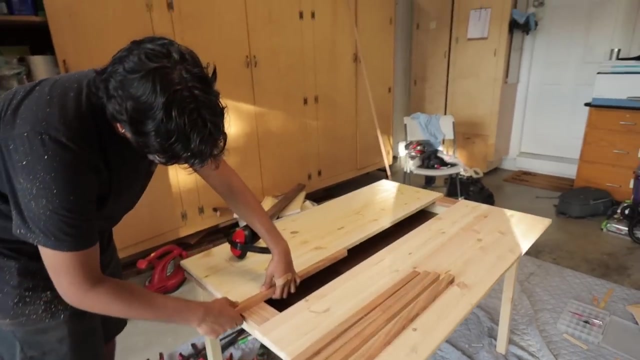 Measure a few times, Cut a few times Sometimes, do whatever you want. really. This is all for Ashton's sake, really. so if you're gonna blame someone, I'd blame him. Right Now we have pieces that are flush here, at least for the most part. 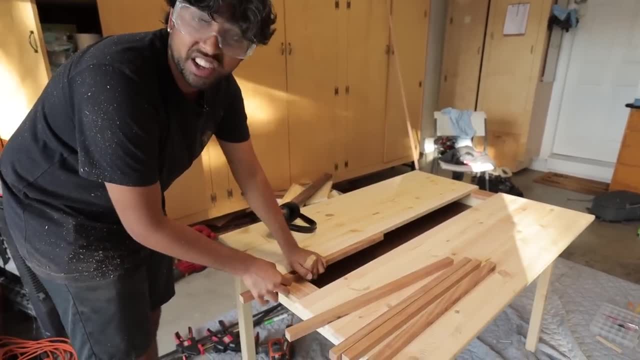 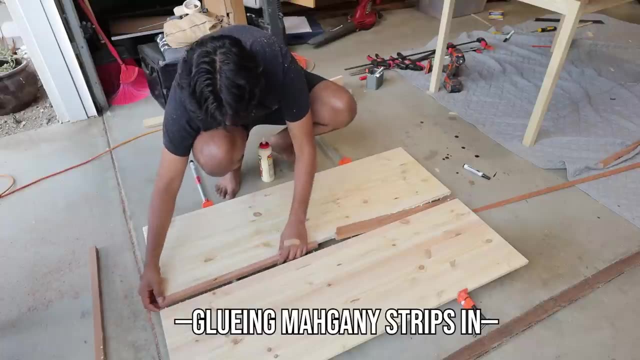 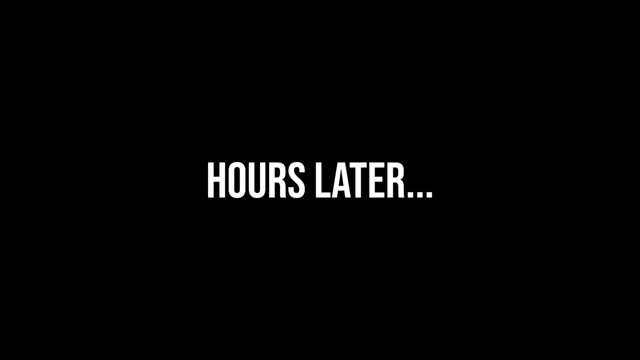 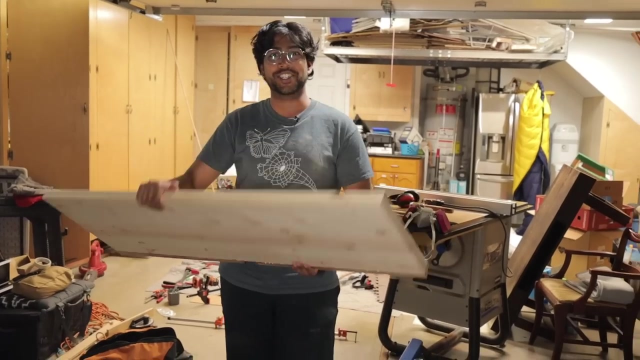 They're a little bit proud, but that's okay. This is a sandable amount. Yeah, Outside of sanding and lacquer we are done Together. it's actually pretty convenient to carry. That's a decent topper system right there. 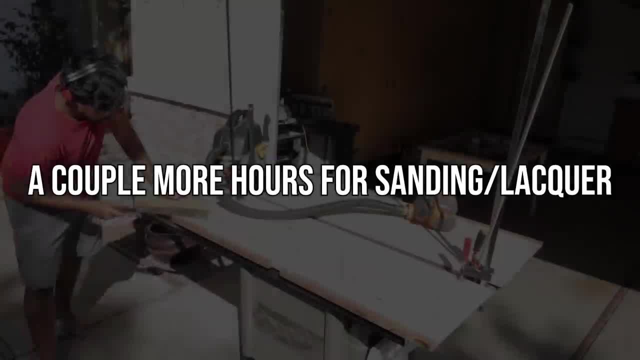 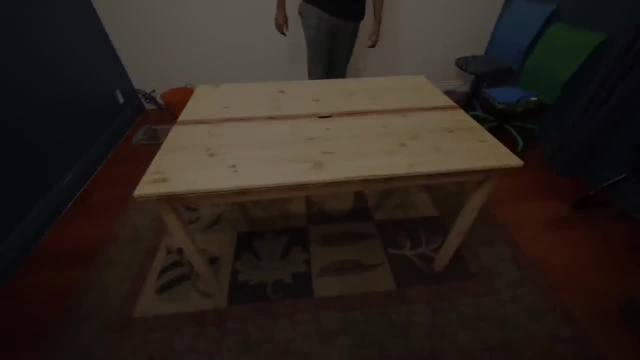 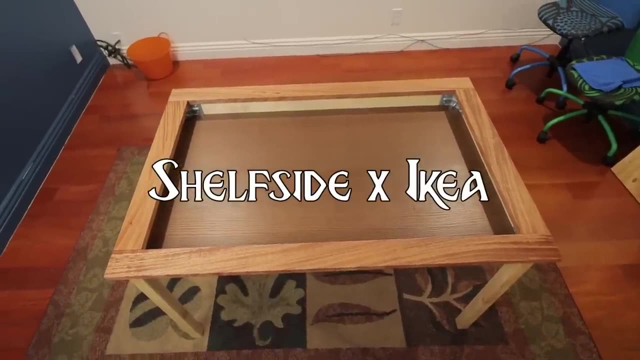 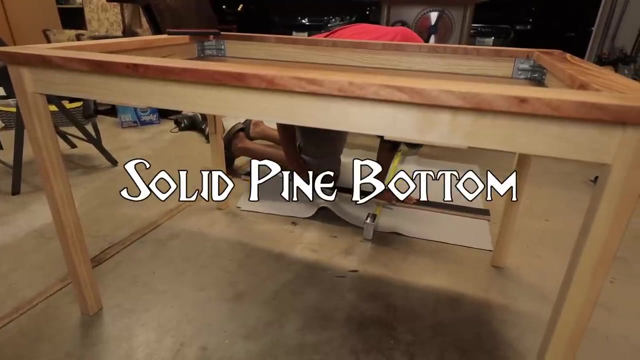 So when you do the gather water action, Yeah, audio's rolling, We're both off. Okay, ready And go. He did it. This is the Shelfside Table 3.0. Our first table that we've made. 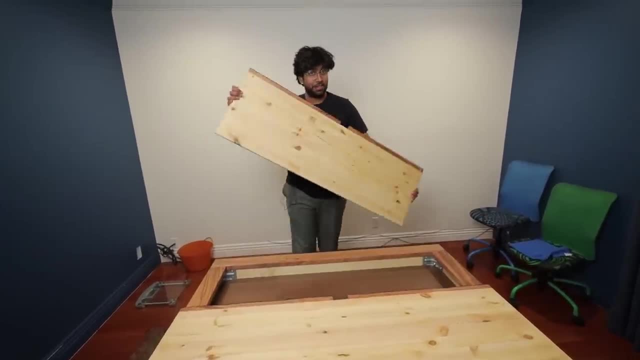 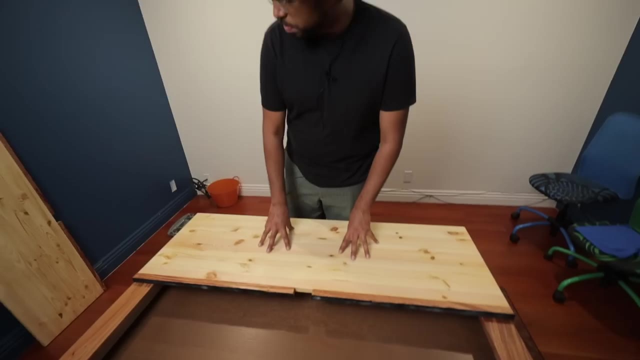 with a topper system that is relatively light. There's no proper alignment system for it outside of just use your eyes and fingers, because it does line up pretty much exactly with the edge. This pine piece and that pine board all used to be one piece together. 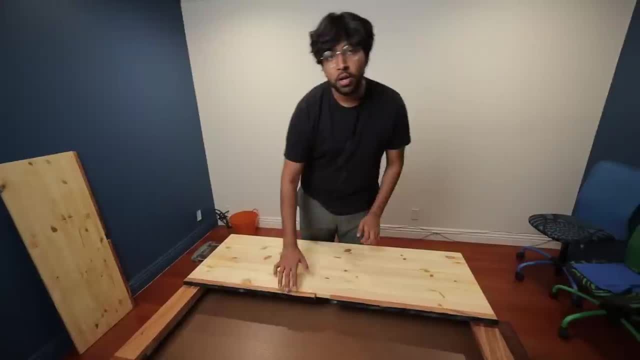 and then we chopped it in half so that we could actually create a proper topper system. We did it at first because we messed up, and then it turns out it just happened to create a really good topper system. A little more work, but yeah. 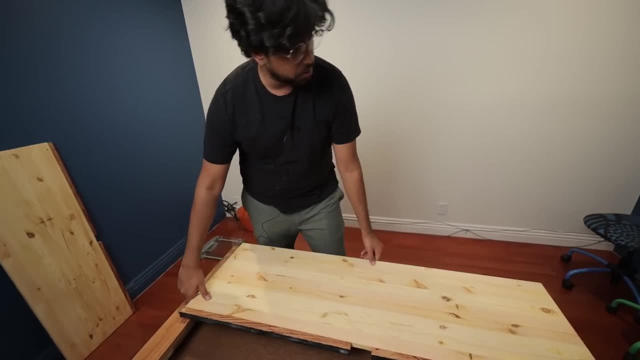 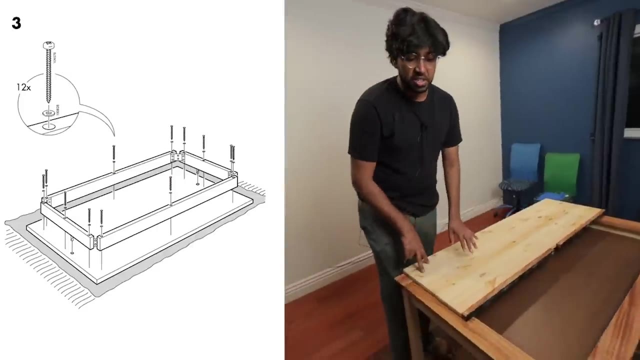 A little bit more work So you can actually see on here on this piece right here. there's a hole right there That actually went to a piece underneath. So the holes that were meant to attach to this piece is what we used to attach the side rails right here. 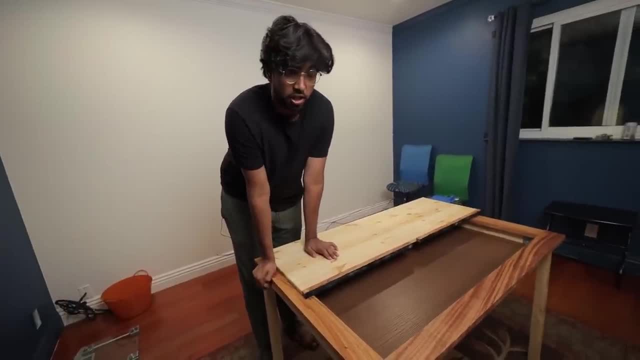 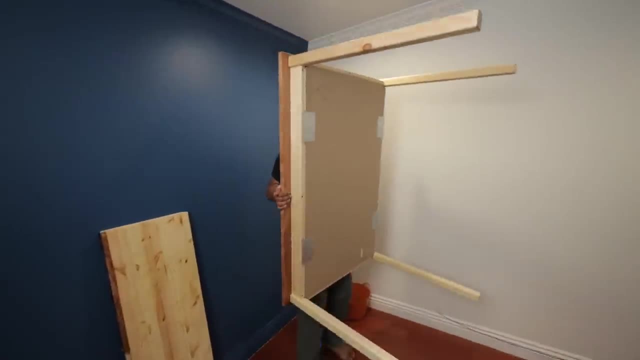 That's why they're actually relatively sturdy. You can lift the entire table off of them. They're held with like three pretty strong and solid bolts. How would we weigh this? Okay, Holy Okay, 263.8.. 263.8.. 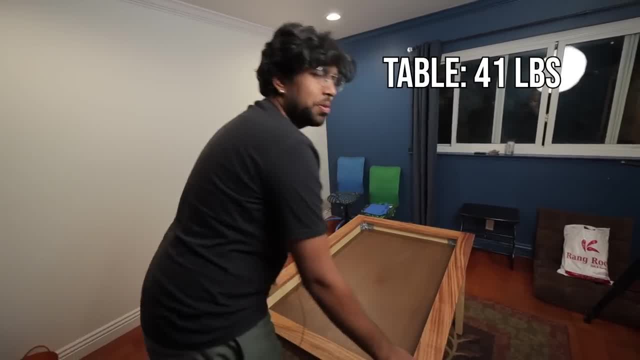 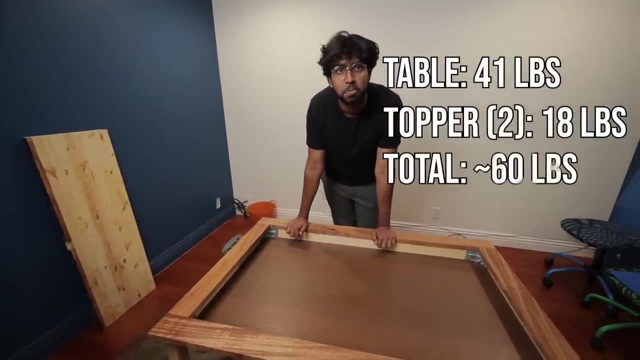 So that's 41 pounds, Right, 222,? yeah, 41 pounds Plus 18 for the toppers, That's 59. Just about 60 pounds total. That's pretty good. And then inside features a two foot by three foot arena. 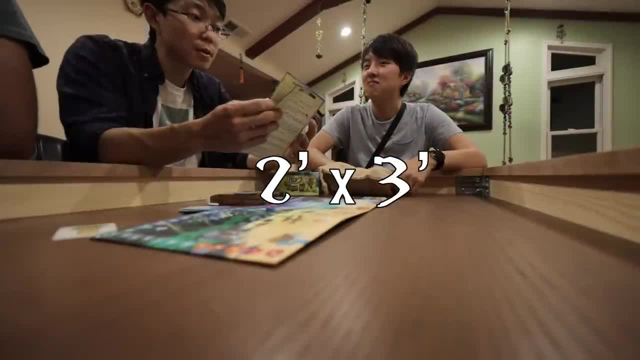 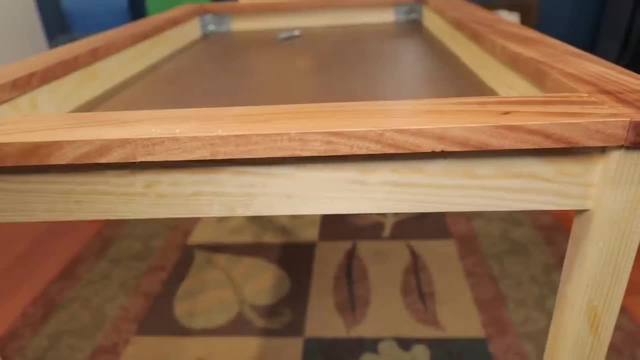 which can play good amount of games. We put a lock bugos on here the other day. Three inch rails right here made out of mahogany. The base is made out of pine which we dissected out of an Ikea table. So this is a bare bones table. 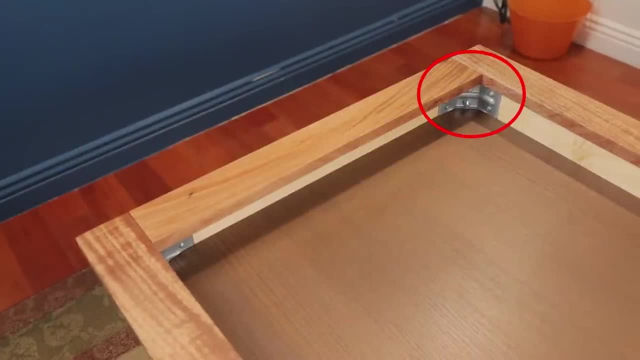 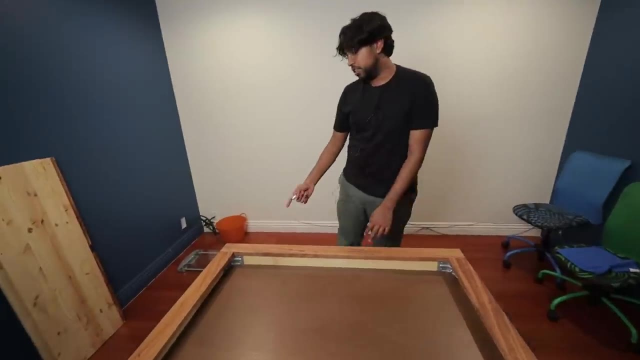 There's no cup holders. You actually see some of the Ikea hardware in there. I left it there because I thought it actually looks kind of cool, but this mounting hardware can be taken apart with this tool, which actually means this table packs pretty flat. 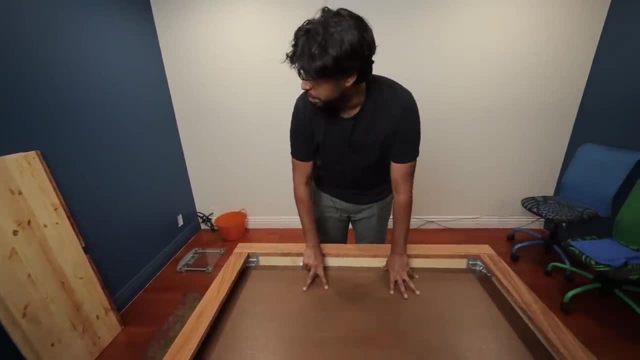 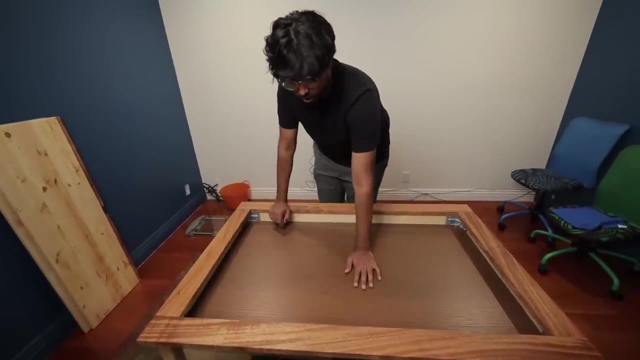 You can take apart the legs, You can leave the legs in here and then you can take the topper, put it on top and it kind of just packs like a flat box. essentially, The actual arena here is all secured pretty well. 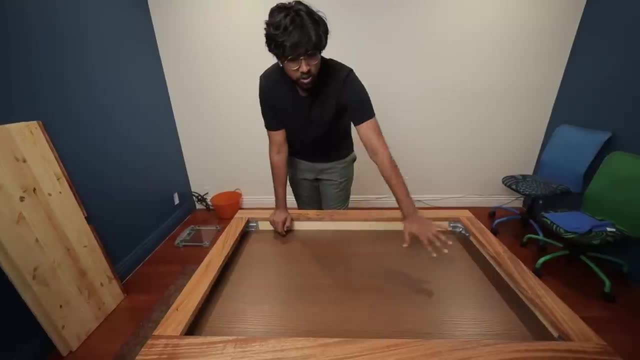 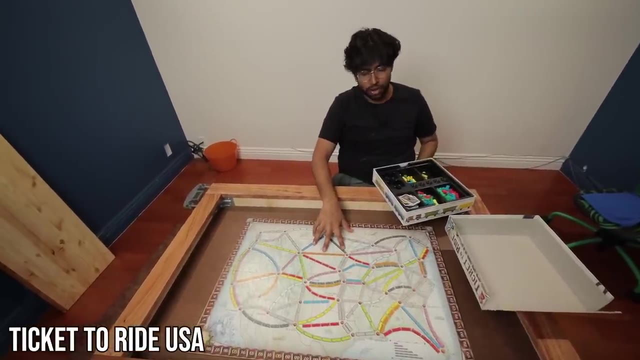 It's made out of MDF- I think about three quarters inch MDF- and it's bolted down underneath using a few panels. There you go. There's not really space for people to have stuff around, though We just put it on the rail right. 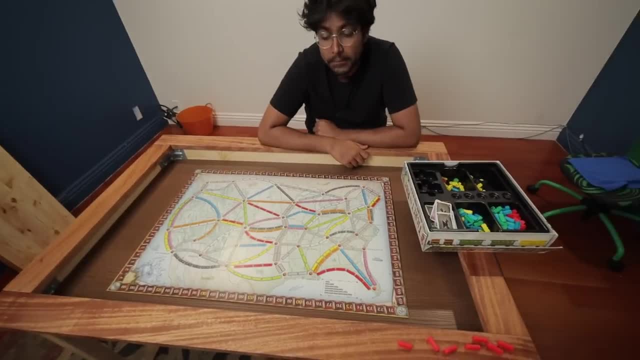 Yeah, we put it on the rail. Yeah, I mean, Catan will fit here fine, right, If this fits. That's true, Catan will definitely fit here fine, which is, I mean, it's kind of like the gold standard, I guess. 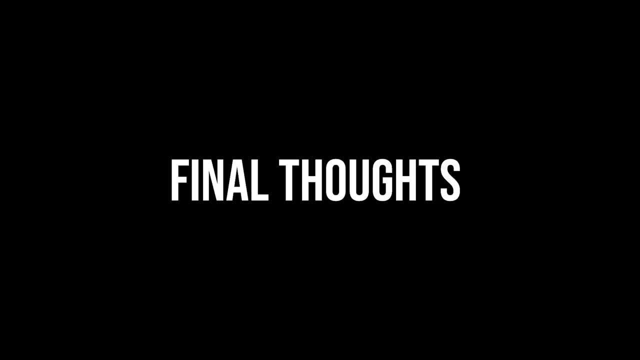 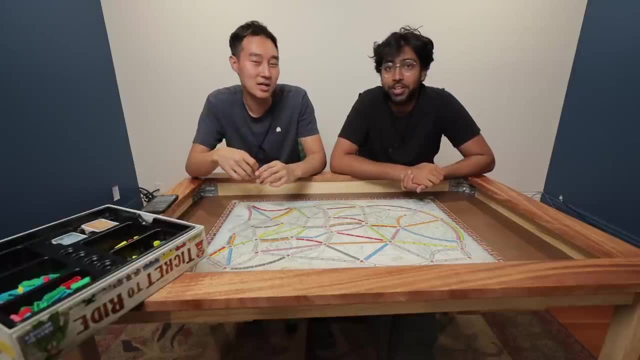 for how small you can go. Catan will fit. We did it, It's here, It fits like it's a ride and it costs us $180? Under 200.. Okay, under 200.. In total, under 200. 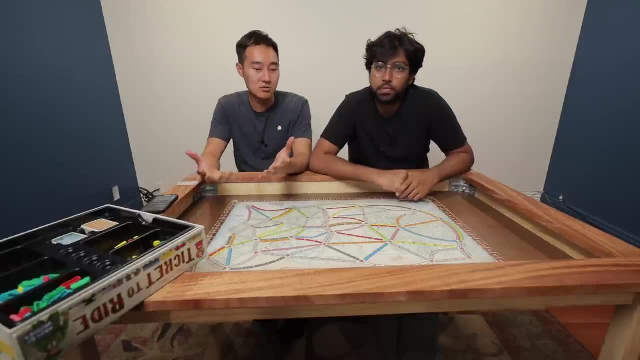 Pranav and I are about six foot. He's a little over six foot and according to the doctor, I'm 5'9". This is a kid's table and it works. Yeah, Yeah, it works. No, it's actually. 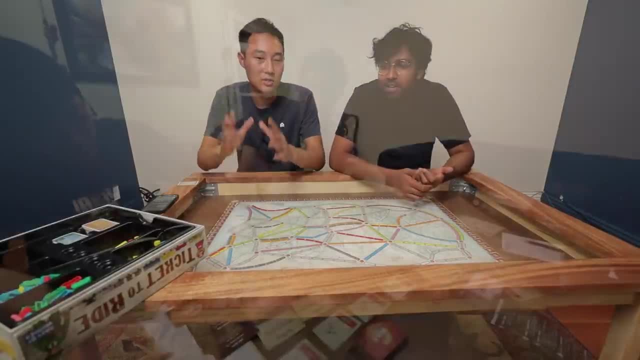 We're sitting here. yeah, It's surprisingly good as a board game table, Yeah, so the crazy thing is that I'll put some footage of us playing on screen. When we were playing, I didn't even think about it being weird. 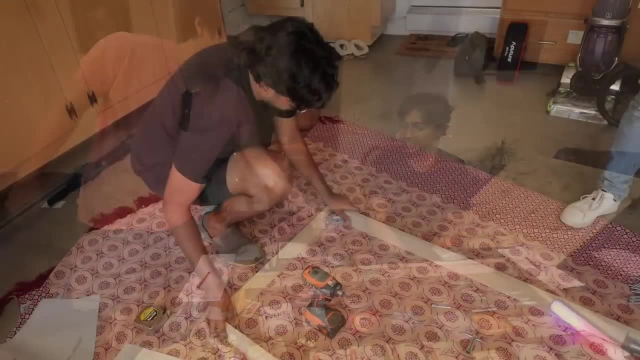 Yeah, right, That's how it was. Yeah, it was just like. oh, we're playing on a board game table, Plus the frame and everything was built by IKEA. I didn't have to sit down and care about stability or anything. 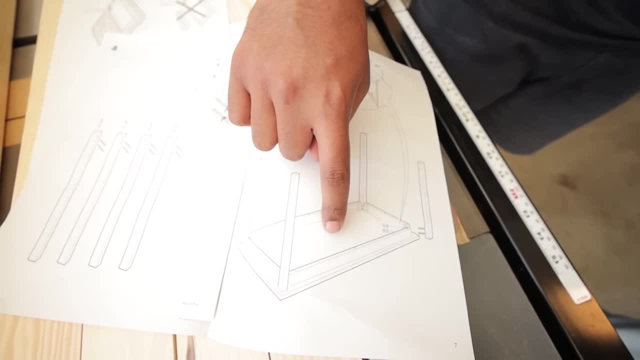 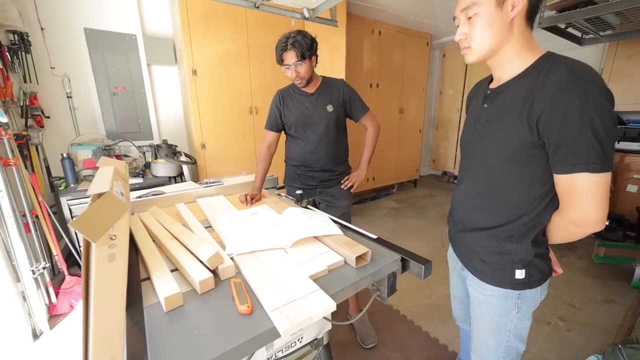 I knew it would be stable if I put everything together. One big thing that I think we've both learned from this is that IKEA DIY projects are a lot easier than doing things from scratch. That's definitely something that I'm going to take to heart from now on. 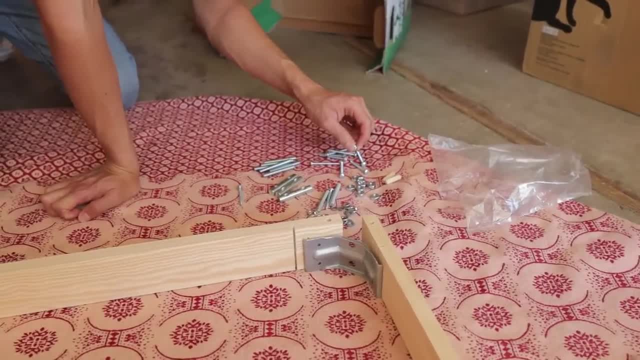 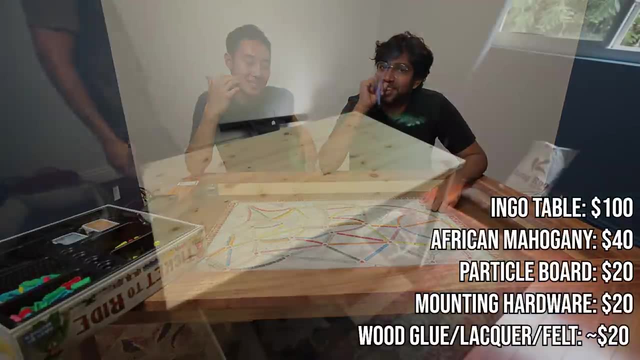 If I'm gonna build something new, I'm gonna try to start with IKEA and then expand from there. I think it's something good to aspire to, but obviously I don't think you'll be following exactly what we did. Don't follow what we did. 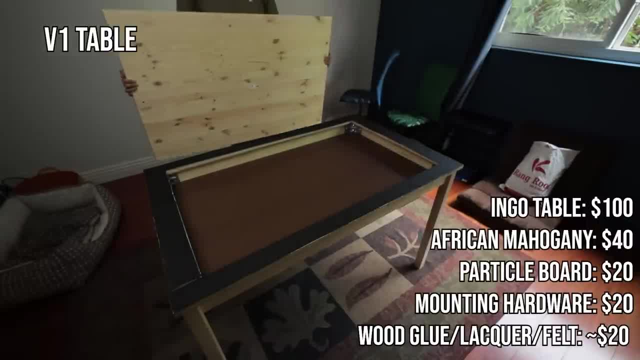 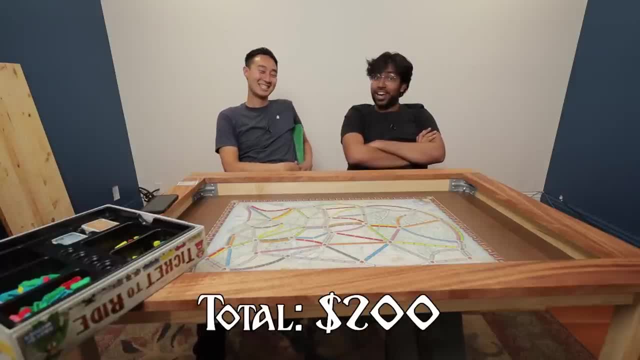 And the V1 table. it works, but you just spend extra time and just get something a little nicer. No injury, no cause to our lungs happened. of course We were very careful. hey, We were very careful, Pretty careful, yeah. 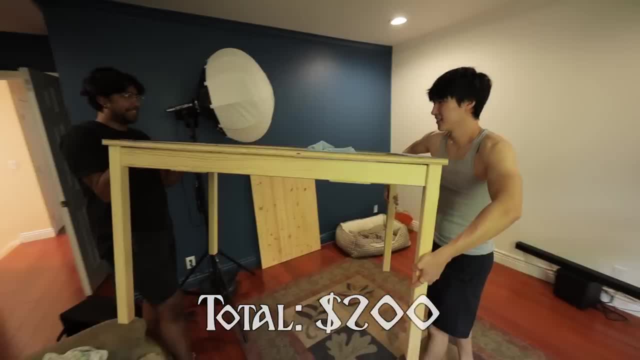 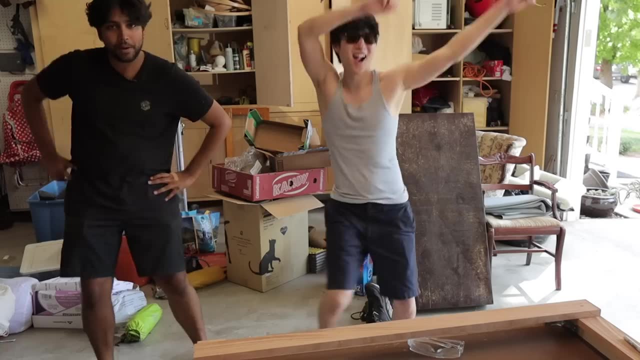 We were pretty careful. We're pretty careful. Ultimately, this was still a lot of work and needed the tools and experience and and, and, yada, yada, but we saved a ton of cash, had some goofs and learned a lot about the potential of IKEA.